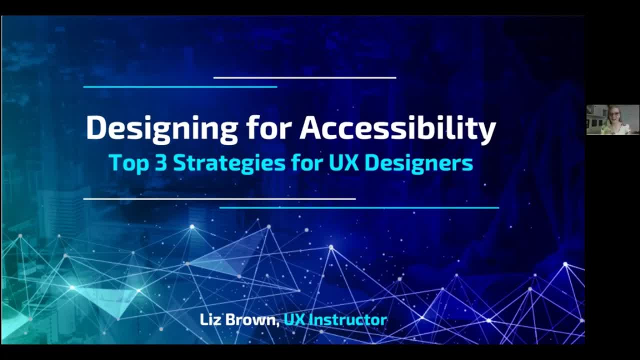 So I'm super excited to talk about this topic. I just love this whole theme of designing for accessibility, So I'm glad that we're going to talk a little bit more about this together and nerd out about this And the cool thing like, as you know, learning to design for accessibility. 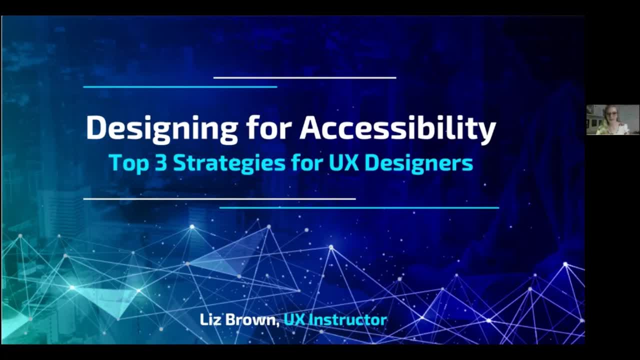 it's a huge leg up for each and every one of us in our careers. It gives you a superior design process And also because few designers are well-versed in accessible design. when you know how to design for accessibility, it makes you stand out as an impressive top tier designer. 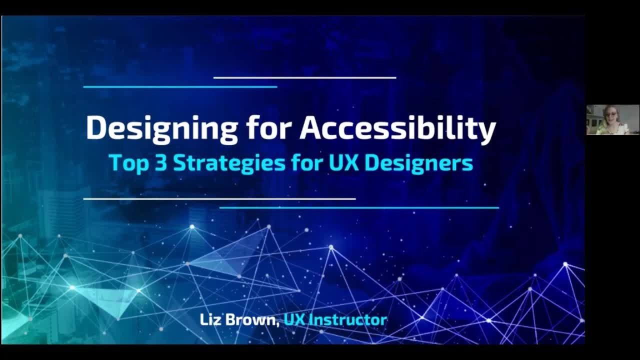 like to your boss, to your clients. But probably the biggest benefit of knowing this stuff is that your team and the client will be will be building better products and be more safeguarded from lawsuits. I don't know if you guys knew that, but because some groups they can actually be. 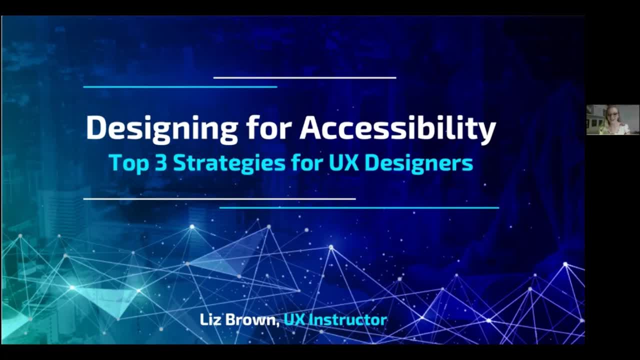 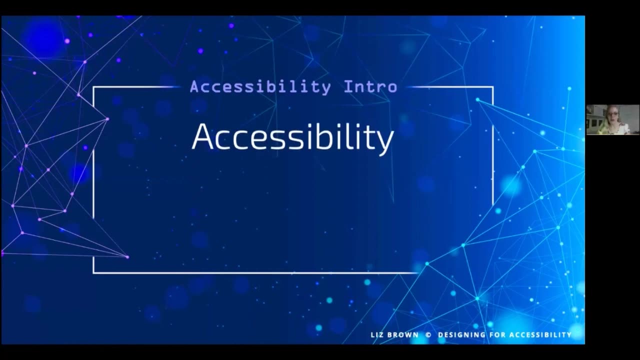 sued for discrimination if their digital products aren't accessible. So let's get into this: The top three strategies every UX designer needs to know about Designing for Accessibility. So let's real quick, get on the same page with the definition. Web accessibility means that people with disabilities can equally perceive, understand. 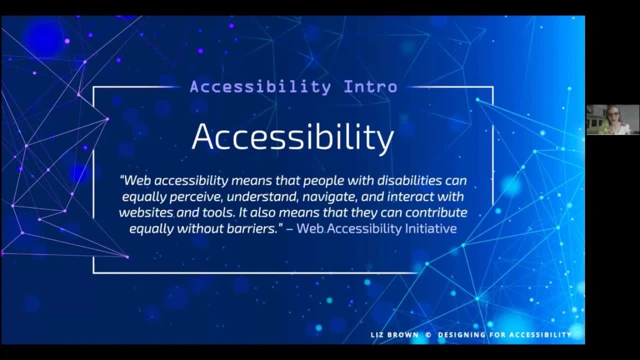 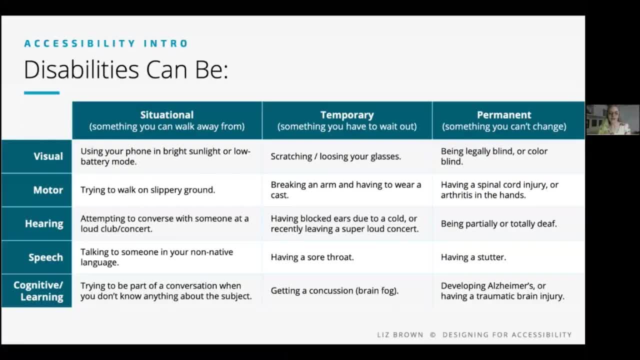 mean to us when we design for accessibility For a lot of us, we think about, maybe, blind people. That's like the number one disability that comes to mind. Right, And yes, blind people are definitely included and they're in this category up. 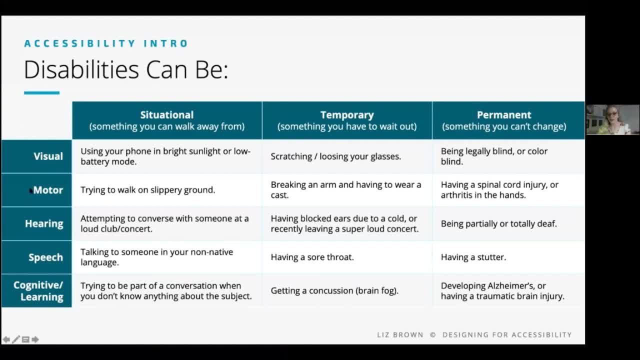 here in visual impairments, but there's also all these other categories: Motor impairments, hearing impairments, speech, cognitive and learning impairments. And the other thing to know is that accessible products benefit people with disabilities as well, and that's because impairments can be situational, temporary or permanent. 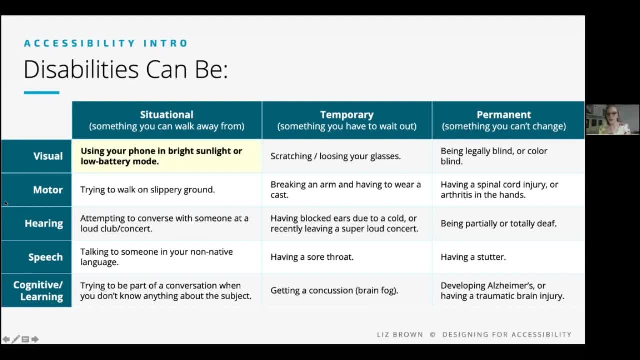 And I'll post these slides after so you can read all these if you're interested. but let's go through just the top row as an example. So in the visual category here, a situational impairment is something you can't walk away from, For example, using your phone in bright sunlight or in low. 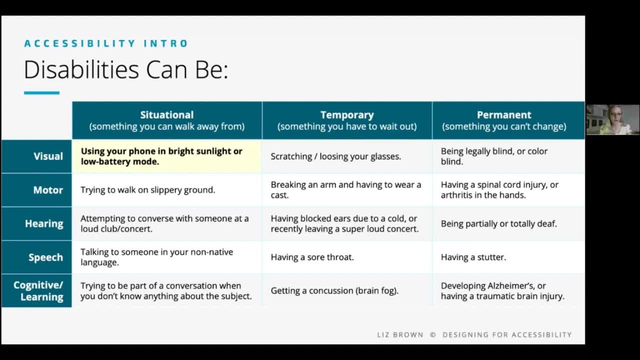 battery mode. there's a glare on it and you can't really see it. so you have that visual impairment, right, But it's situational, You can walk away from it. You can go inside and fix the issue. A temporary disability is something that you have to wait out. So, for example, you scratch your. 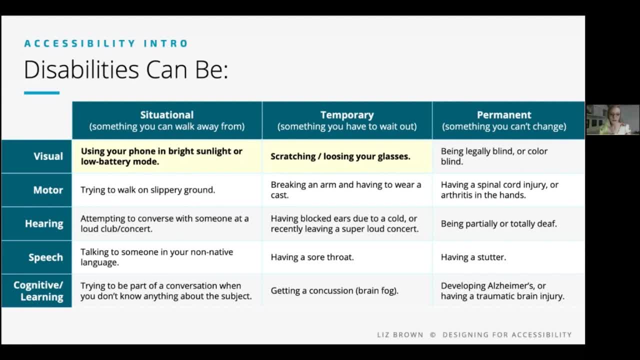 glasses. You have a vision impairment now looking through the scratched lenses, but it's temporary. In a couple of days or whenever you get around to getting new glasses, that is no longer an impairment for you. And then an example of permanent disabilities is like being legally blind. 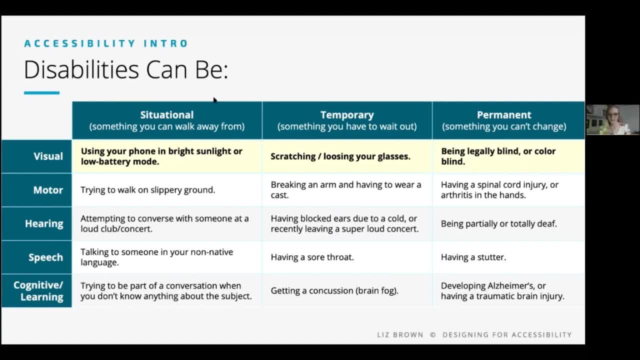 or being colorblind. You can't change that. The thing to remember is that accessibility is usability for all, And I really love that. That's like a really poignant definition of it. I think Usability for all meaning it's for people of all. 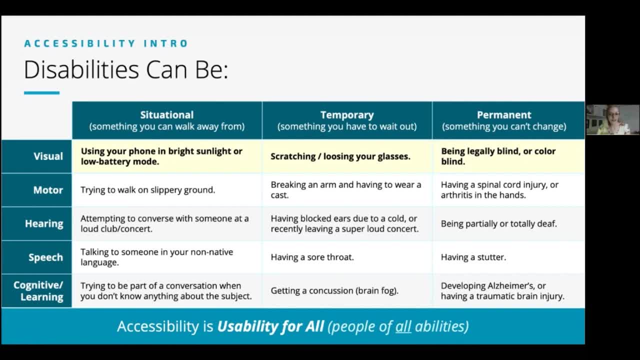 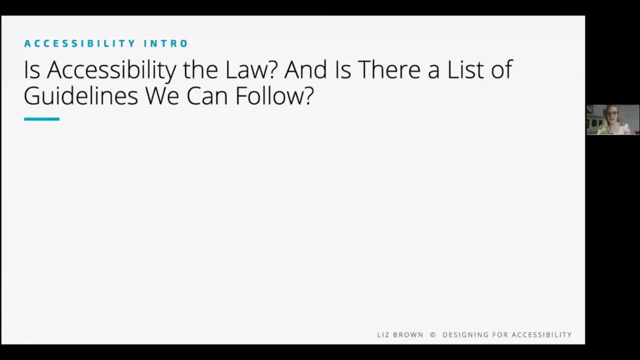 abilities. A question that often comes up is whether or not accessibility is required by law and also whether or not there's some standardized checklists of rules that we can follow to make digital products that are accessible, And I think that's a really important thing to remember. 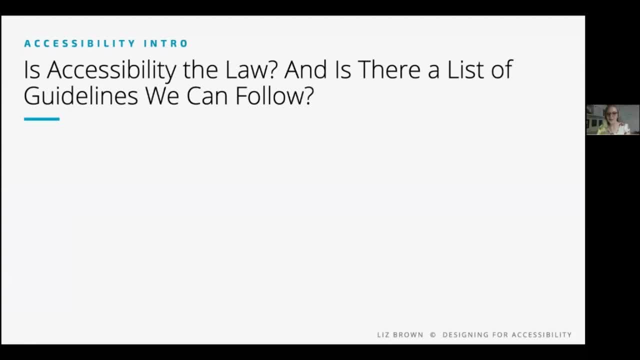 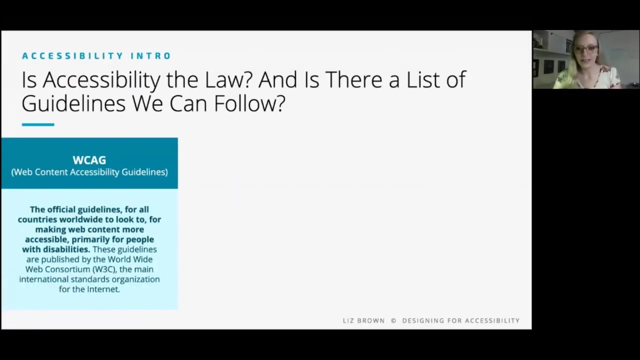 And the answer to these is yes and yes, But let me explain. So, when it comes to accessibility compliance, there's two main things that we designers should know about. So the first is the WCAG. Well, that's the Web Content Accessibility Guidelines. So they're the or some people like. 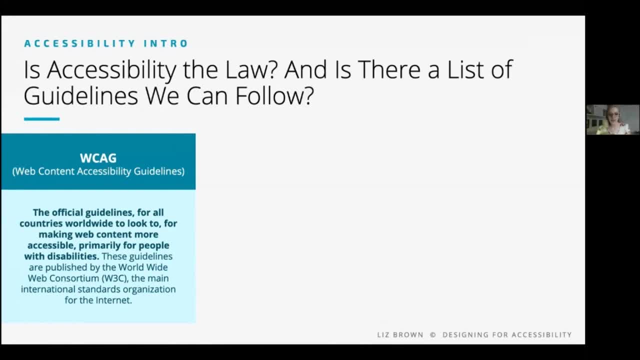 to call them WCAG, And it's the official set of guidelines for all countries worldwide to look at to make their web content more accessible. And it's the official set of guidelines for all countries globally, primarily for people with disabilities, And these guidelines are published by the. 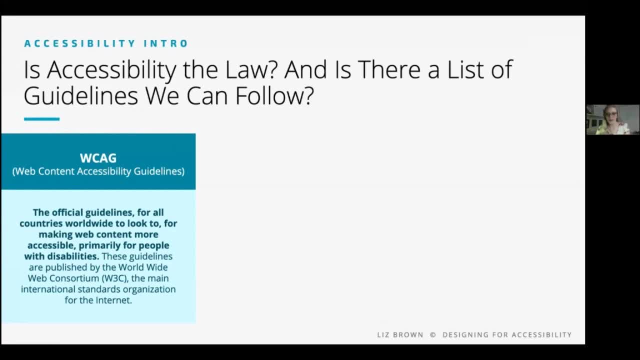 World Wide Web Consortium And that group is the main international standards organization for the internet. So the WCAG, that's the golden set of guidelines for us designers to follow. That's, or for us digital product creators to follow. That's like the list And anyone who 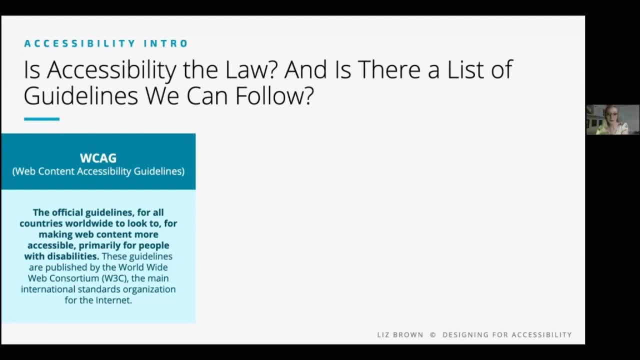 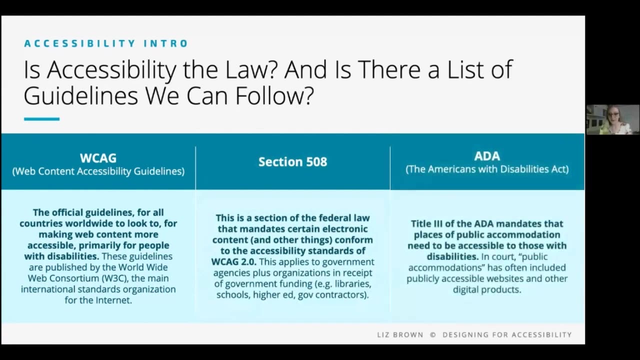 knows anything about accessibility is going to know about WCAG most of the time, because that's the list they're following. The second thing that we designers should know about is our country's laws that allow it to enforce digital accessibility. So for us here in the United States, those laws are Section 508 and 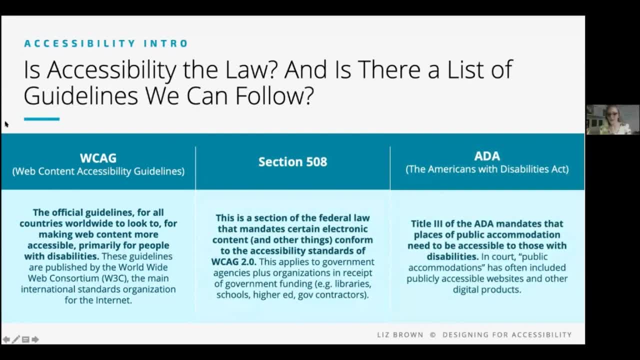 the Americans with Disabilities Act, Section 508, that's the section of the federal law that mandates certain electronic content be accessible- So websites, apps, PDF- and it mandates that they conform to WCAG 2.0. And this applies to government and federal law, So it's a section of the federal. 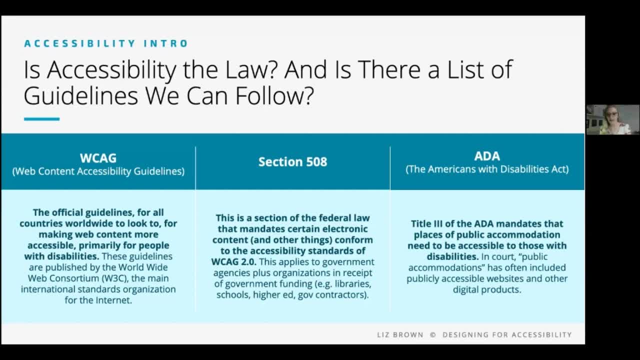 law that mandates that they conform to WCAG 2.0. And this applies to government agencies plus organizations in receipt of government funding. So that could be a lot of things right: Libraries, schools, some higher ed and certainly government contractors. So anything touched by. 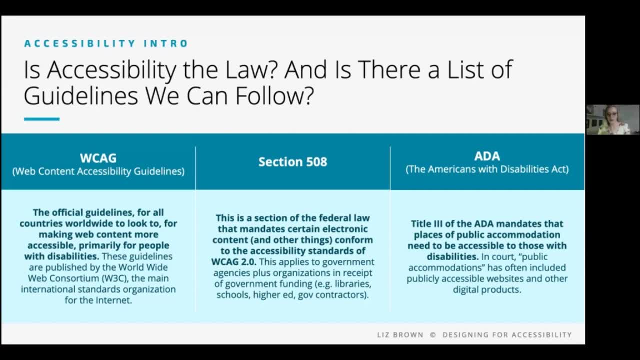 government money. So if we're working on a project that's for a group associated with government or receives government funding, we're legally we're going to be legally mandated to follow Section 508 and make it accessible and make it comply with WCAG. And that's how a lot 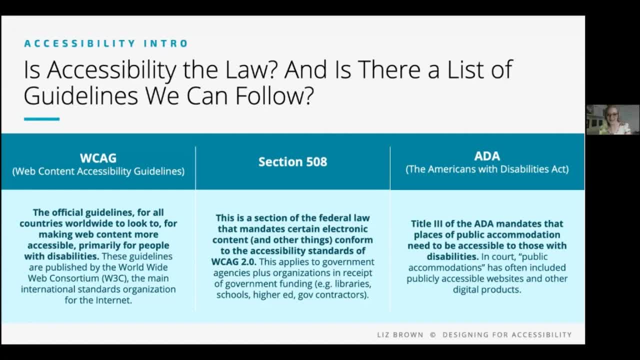 of countries do their laws. The law says: make it accessible, but then they point or reference to the WCAG as the list for people to follow to actually achieve accessibility compliance. So a lot of countries do that. Okay, so that's for like. 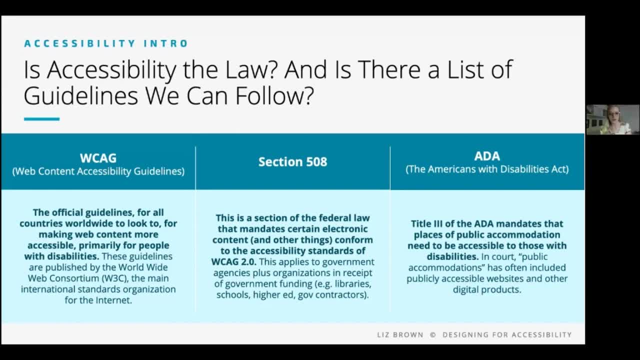 government stuff Now non-government stuff. The law that most often applies in that case is the ADA. So Title III of the ADA mandates that places of public accommodation need to be accessible to those with disabilities. The verbiage in the ADA is that places of public accommodation need to be. 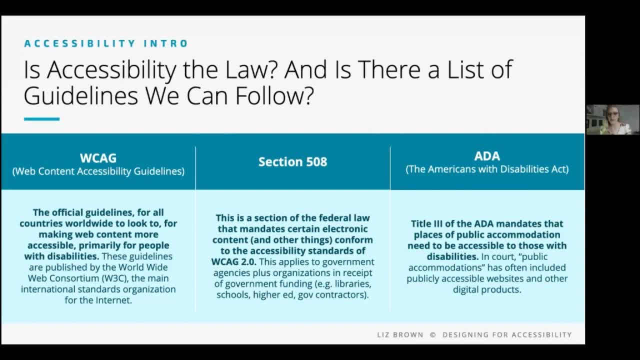 accessible to those with disabilities. The verbiage in the ADA is not totally explicit about what public accommodations includes, But many companies have gone to court because their websites weren't accessible And in court it has been ruled that public accommodation most often includes: 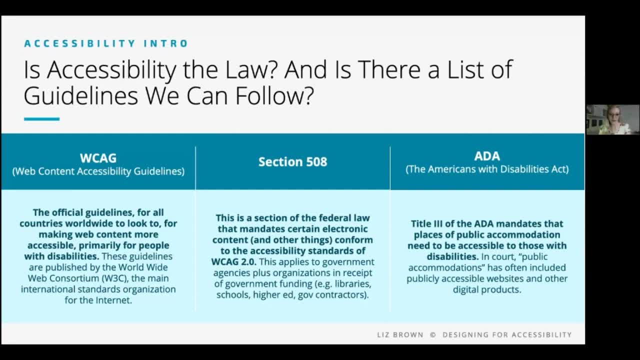 publicly accessible websites and other digital products. Long story short, if our project isn't caught in the net of Section 508, then it will likely be caught in the net of ADA. So that's why I say we're going to have to make it accessible And I'll see you soon. 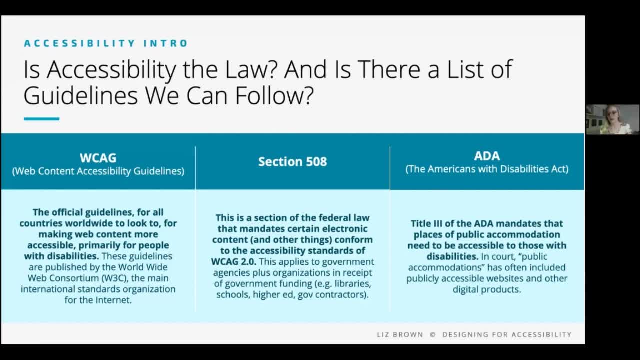 that accessibility is the law, But really we want to make our digital products accessible simply because it's the right thing to do And, you know, accessibility becomes easy when we make it part of our standard default UX process. All right, that was the quick and dirty accessibility. 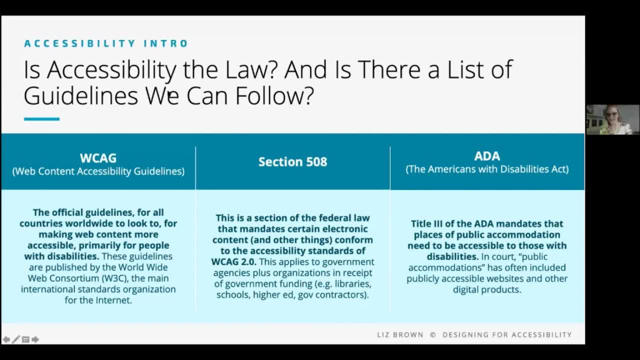 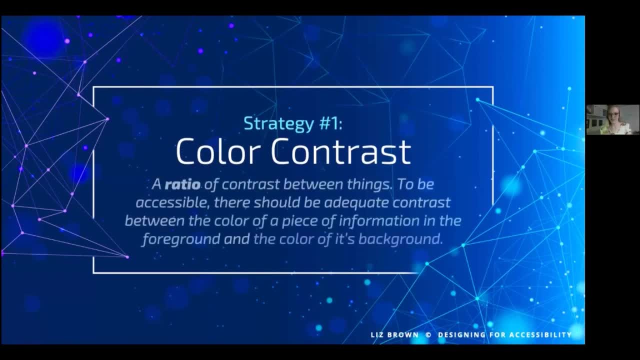 101.. Now let's get into the good stuff. Let's get into strategy number one, and that is color contrast. So, starting with a quick definition, Color contrast is a ratio of contrast between two things To be accessible, there should be adequate contrast between the color of a piece of 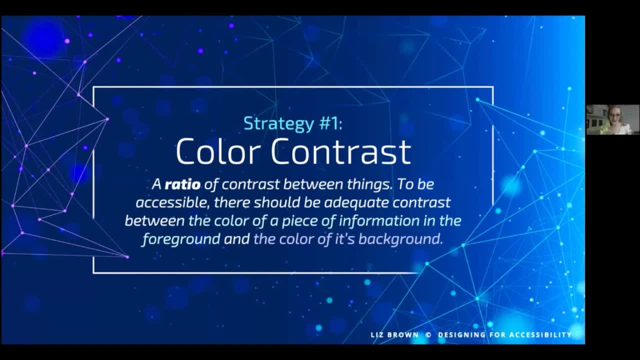 information in the foreground and the color of its background. Now you might be thinking, Liz, color contrast is so elementary. Everyone who even knows a little about accessibility knows about color contrast. Well, let's play a little game and see what that is. 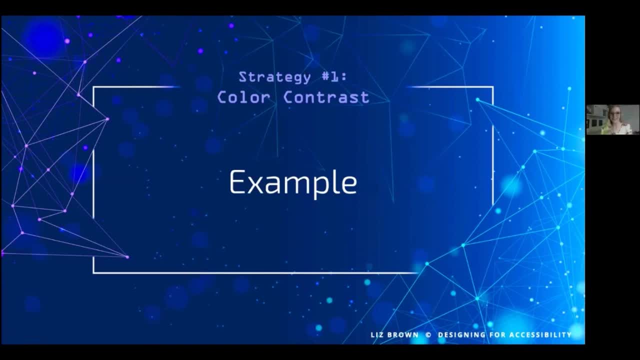 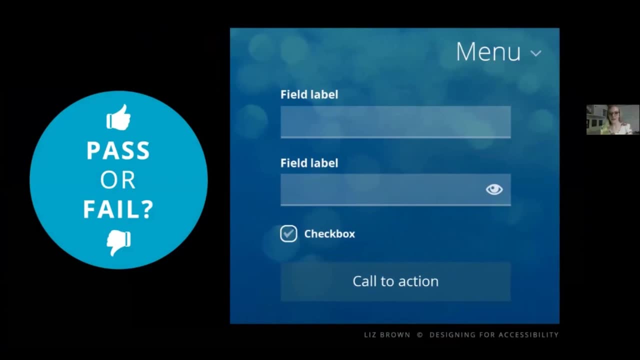 see with an example here and see if we find any surprises. so take a look at this mock-up in regards to being color contrast compliant. does it pass or fail? so give me a thumbs up or a thumbs down to the camera. so thumbs up meaning all the essential stuff looks to have adequate contrast. 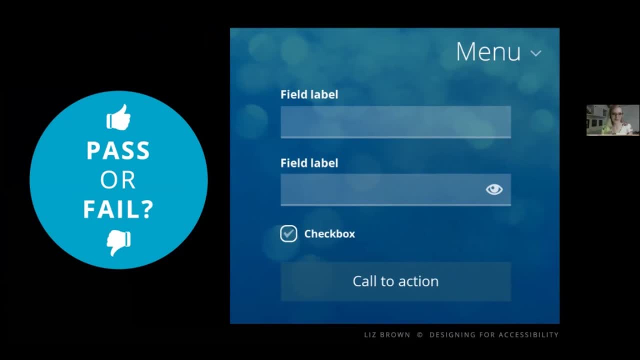 thumbs down means there's not enough contrast. what do you guys think? i'm seeing a lot of thumbs down. all right, cool, okay, so i'm not going to give you the answer quite yet. we're going to come back to this in a minute, though, but first let's learn how to achieve. 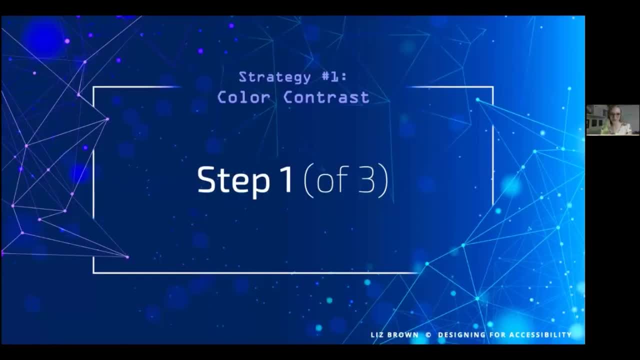 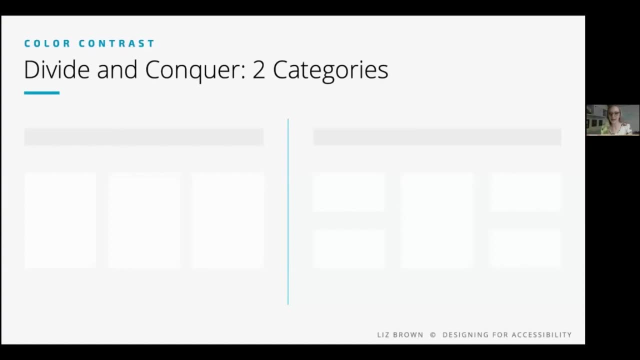 strategy number one. so there's three steps and step number one. we're going to mentally put our interface elements into two categories. so the first is information bearing elements and the second is information bearing elements and the second is decorative and disabled elements. so we're not like physically moving. 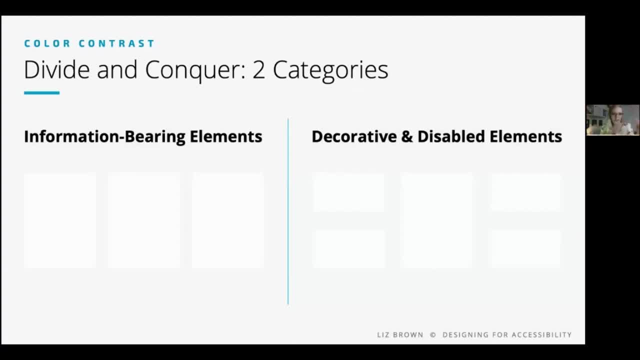 our ui elements into two categories. you just kind of look at your page and decide, okay, that's information bearing, that's decorative, that's information bearing. so in the information bearing category, that includes text, including images of text as well, plus their various states, hovered, focused, selected, as well as standalone icons. so standalone icon, meaning the icon doesn't. 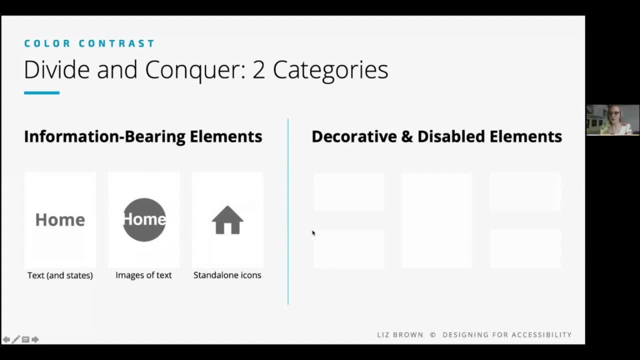 have a text label next to it. the weight of conveying that information bearing element. that information is on that icon to do all on its own. and then decorative and disabled. that includes disabled buttons, check boxes, sliders, radio buttons, plus decorative things like a background pattern, an artistic border, things that like, if you couldn't see them, it's not a really big deal, you're not? 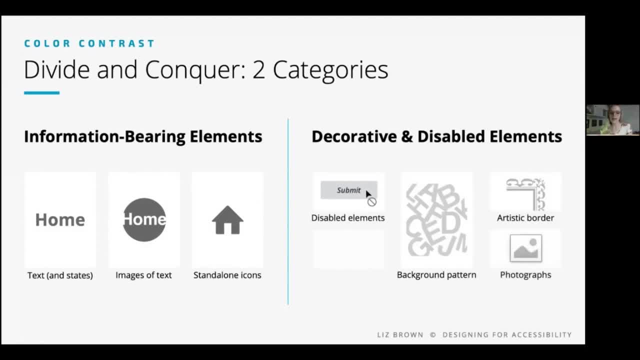 losing out on any information. also in this category are photographs and logos. now, both of those do convey meaning, but, like for photographs, no one could expect a designer to change the contrast between. like you know, if it's a photo of a dog in front of the sky, you can't change the contrast. 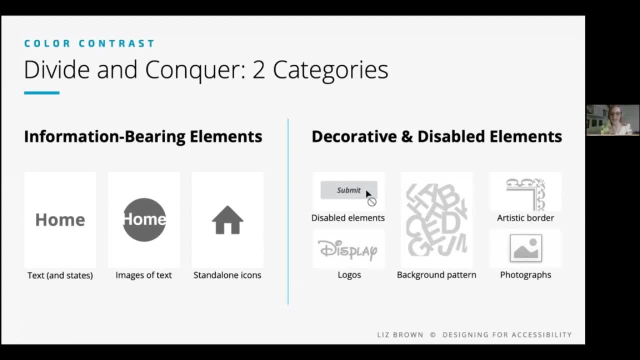 between the dog and the sky. so that's why it falls into this category. plus, we have alt text to convey the informational part, and then logos. it's in this category because, like, say, you're doing a website for coca-cola, you're not going to change the coca-cola red to be darker or lighter. 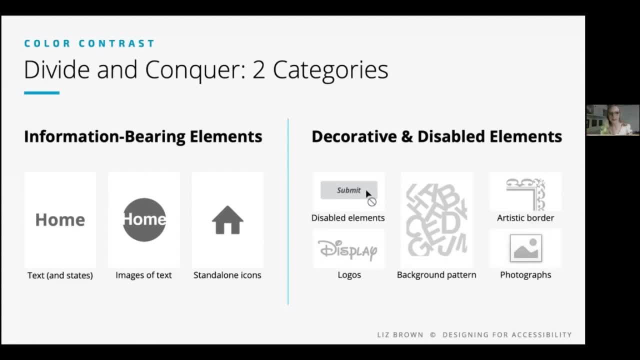 to pass color contrast. that would be like against their brand standards and go against their whole color palette. right? so you don't really want to mess with people's branding, so that's why that's in this category as well. all right, so once you've figured out which of the two categories 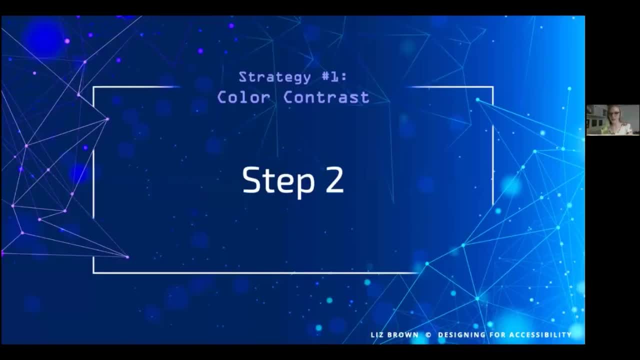 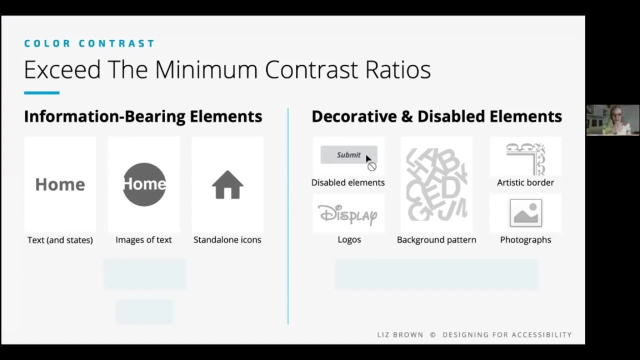 all your ui elements fall into. then we move on to step number two, which is to then meet or exceed the minimum contrast ratios for each category. so since not everyone has 20, 20 vision or giant retina monitors, we make all of our information bearing elements have a contrast ratio. 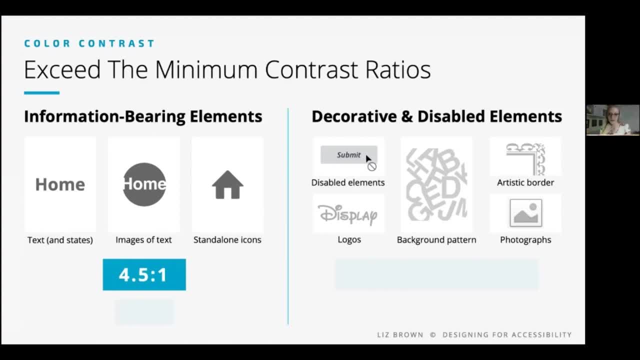 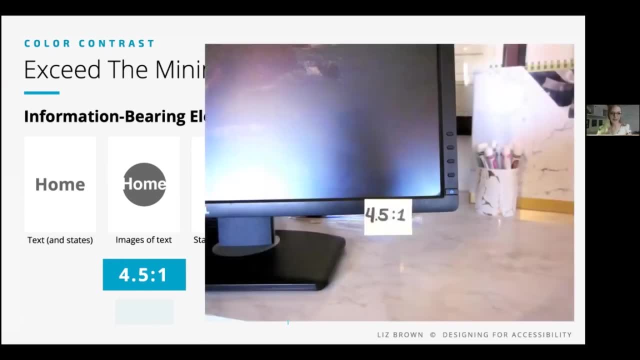 of at least four and a half to one. so these are minimums. so what i did to remember this when i first started is i put a sticky note on my monitor that said 4.5 to 1, so i didn't keep having to look. 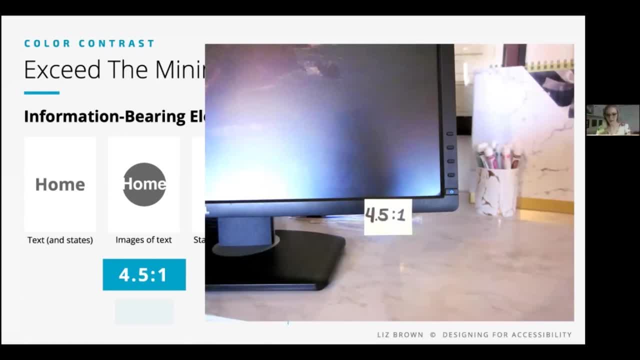 it up, because when you start designing for accessibility, or if you're already doing it, this is like the golden number. you reference this number a lot, so consider putting a sticky note on your monitor. so there is one exception to that 4.5 to 1 rule, and that is that you're going to want to. 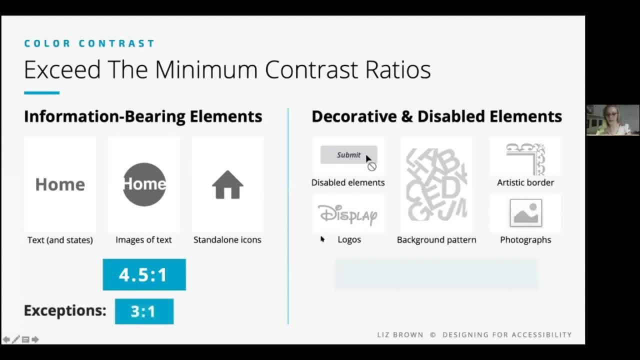 put a sticky note on your monitor and that is for a few things: large text, graphical objects and ui controls. so for them the contrast ratio falls to three to one. we're going to look at those here in a minute. for decorative and disabled elements, what's the required contrast ratio? does anybody? 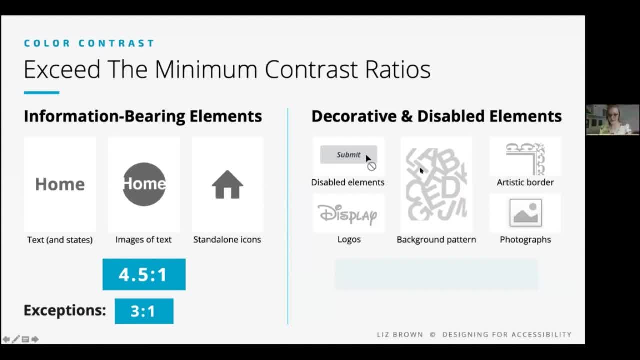 know, okay, so i'll just tell you. if you were going to say there isn't one, you would be right, but you're going to want to remind you that this does not apply to a variety of other disabilities, but there are a number of other elements here, and being able to know what they are using. 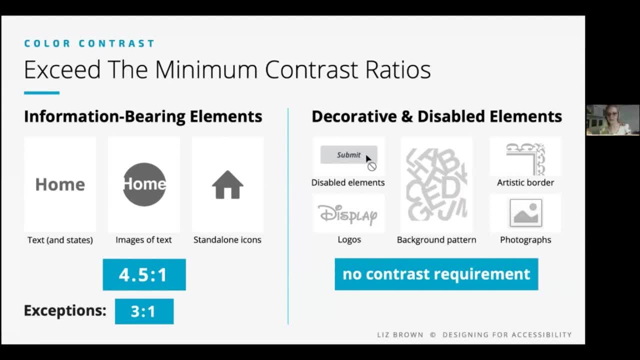 and how you can use those is not fair, and the reason i'm showing you some of those is because they only display these elements by their size and they are available by their color. so i'm going to explain this to you and then i'm going to show you some of them in a minute. 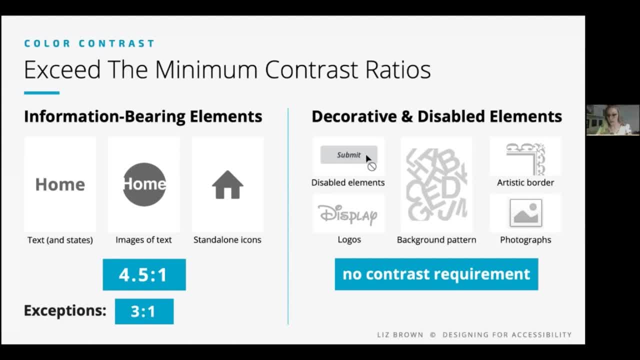 all right. so what i'm going to do here is i'm going to go back to the last slide for me, and i'm going because there's a reason. we don't just delete the button when we disable it, right. We don't just leave a blank white space, We leave it there, but we gray it out because we want people to still be. 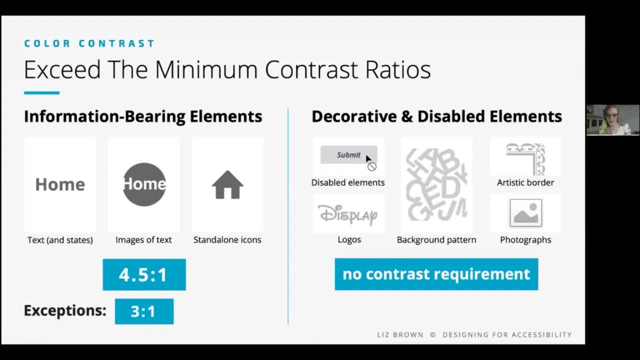 able to see it and to read it and know that it's just not clickable, right. But really all it takes is a tiny bit more of our creativity to make it contrast compliant and still disabled, looking Like this example here. this one is contrast compliant but it still looks disabled, So it 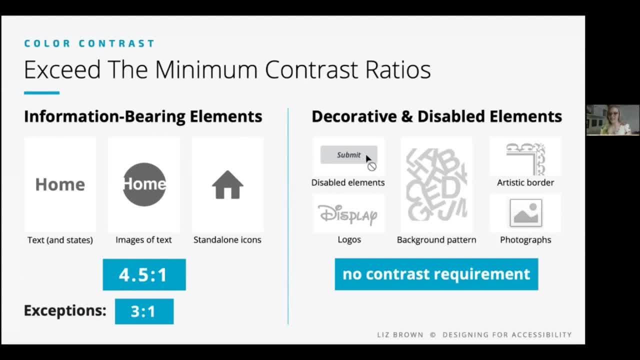 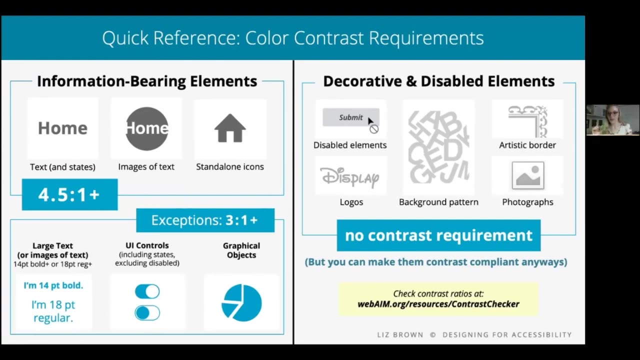 can be done. All right, let's talk about those exceptions down here. So I'm going to squeeze those exceptions onto this slide right here so we can see everything together. So those exceptions are large text, UI controls and graphical objects. And now, if you want to, 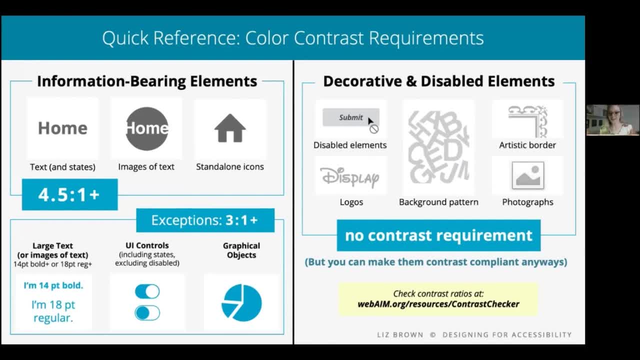 you can screenshot this slide, because this is your quick reference guide to color contrast. If you can memorize this one one slide- that's why I shoved it all on here together- If you can memorize all of this, you will be leagues above other designers who don't know how to design for accessibility. 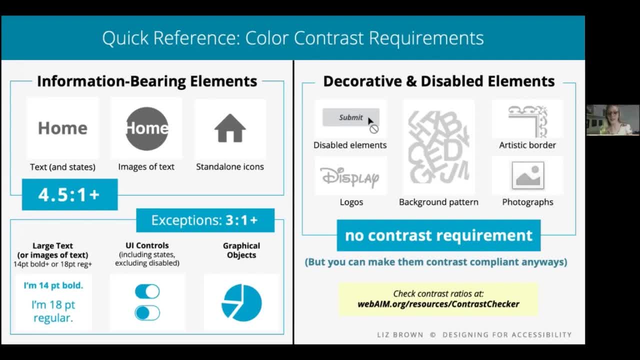 This is like the almighty cheat sheet for achieving color contrast compliance Because, like, if you think about all the math tests we've taken, the grammar tests we've taken, in comparison this one slide isn't that much right. So yay for wanting to be better designers. 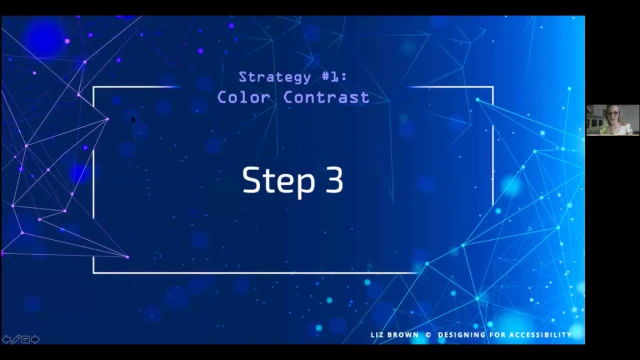 Okay, we have one more step to go. So step number three. So now that we know- we actually know what color contrast is, we're going to go ahead and do a little bit of a recap of what is needed, how much, how many, what is required and what the required ratios are. 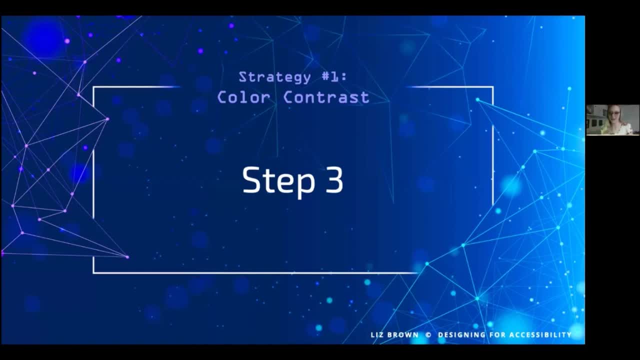 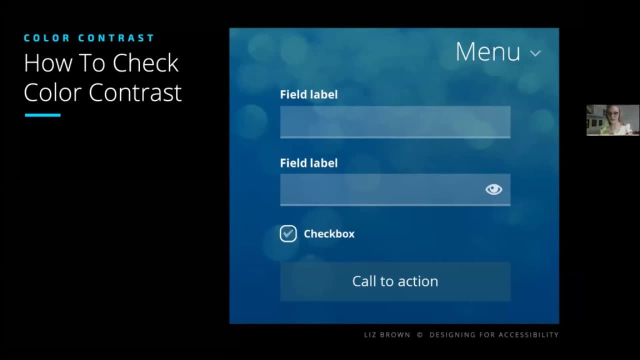 Let's put that knowledge to practice and make our UI designs contrast compliant. How do we check for color contrast so we can achieve these ratios? So I'm going to just real quick show you. there's a lot of online checkers that you can go to, but WCAG. 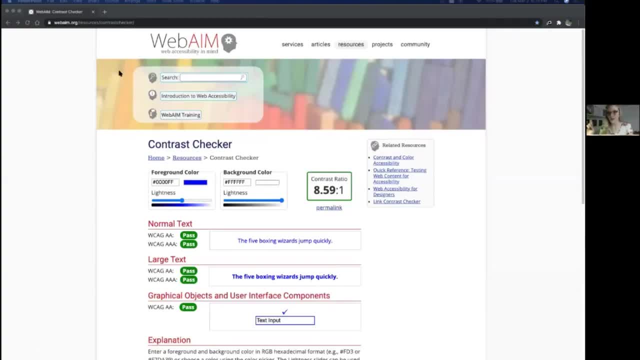 I mean a WebAIM. Can you see, okay on the screen? do you see the WebAIM website? Okay, cool. So this is my favorite website just because it's a trustworthy source, source Like: if anything in the WCAG changes, I know that they'll update it here, For example. 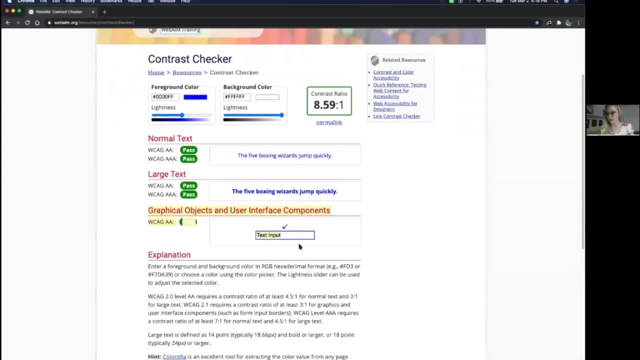 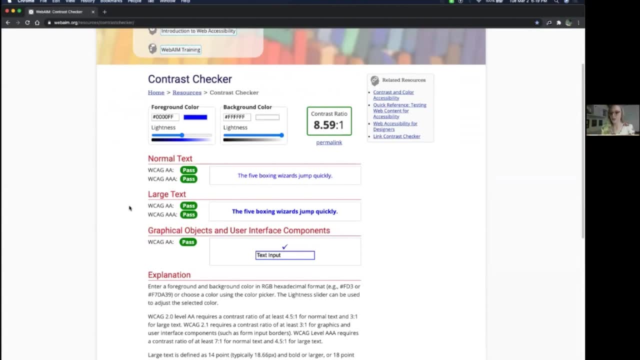 they just. the latest thing they added was this section down here, because WCAG got updated, So they updated their contrast checker tool. So I like this site just because I can. it's a trustworthy source, but there's a bunch of other more snazzy tools out there too. So if I'm going 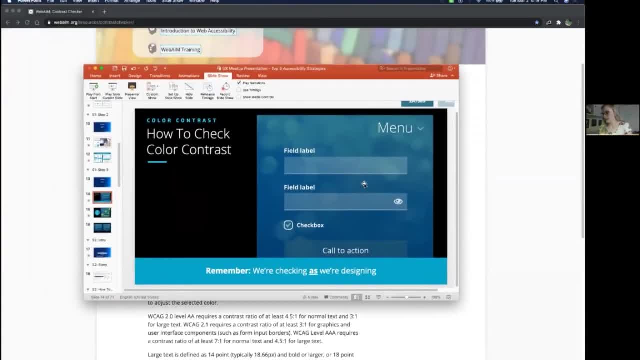 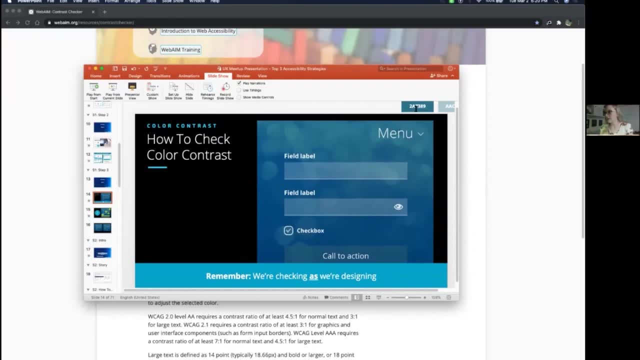 to check this little UI here that we were looking at. okay, say that, starting at the top. say we're going to check the word menu, So that's white And then the background color. I already eyedroppered the hex code here. So you grab the hex code. whoops, you grab that hex code and then you 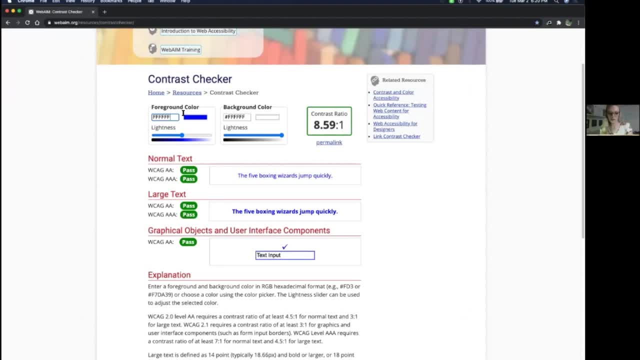 paste it in here. So my foreground, that was white And then my background. I paste that in. So now this is what you look at. 5.3 to 1 is the contrast ratio And if I slide this slider here, 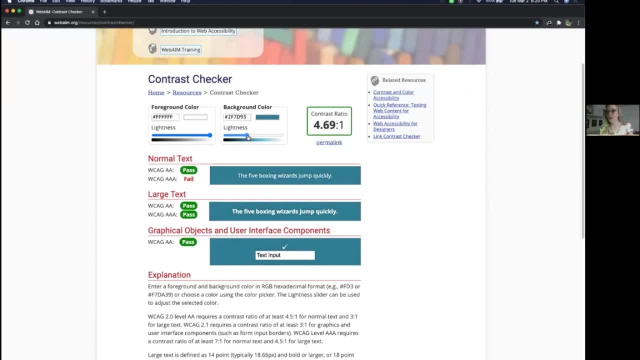 you can see how that number changes. So this is how you can get the contrast ratio that you want And say, for example: I don't like you know, if I darken, I don't really like it. You can click on these little swatch icons too and like: make it a little. 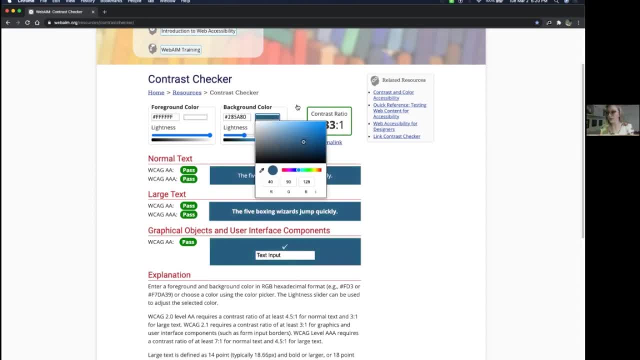 more cobalt if you want to get the to get to the color you like, And then also, as you're sliding, you can see these things pass or fail down here. So you want it to get to pass for the category that you're looking at. The difference between AA and AAA is that AAA is more stringent, So 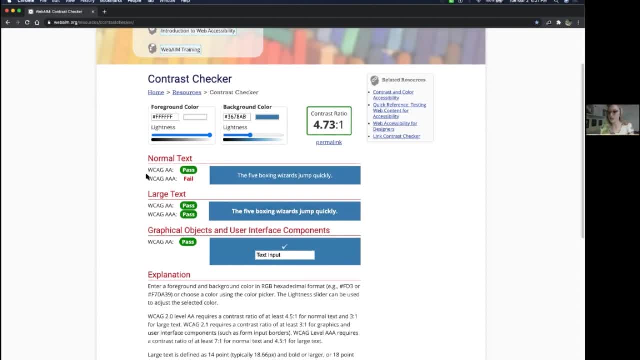 sometimes you might have a contract specifically like government contracts, or you know certain things that are required to be super accessible, like for sure accessible. So WCAG has the AAA for instances like that, But for the vast majority of us, the majority of the time, 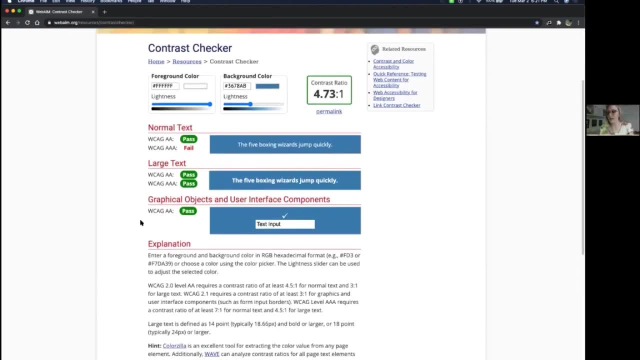 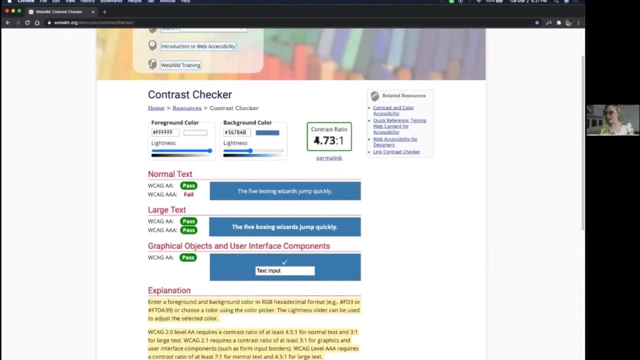 we're going to be looking to pass on the AA criteria And if you forget all this stuff, WebAIM is really nice And they explain all of it down here for us. So that's how you check to make sure you've exceeded the 4.5 to 1. 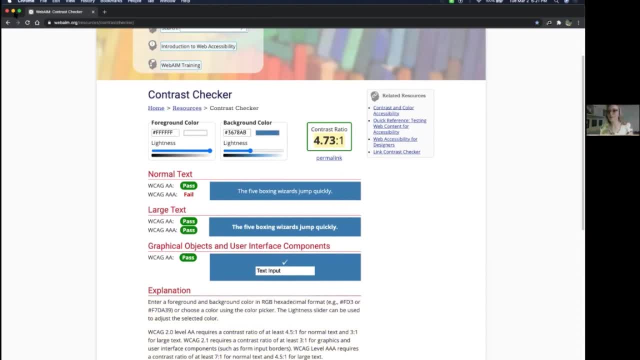 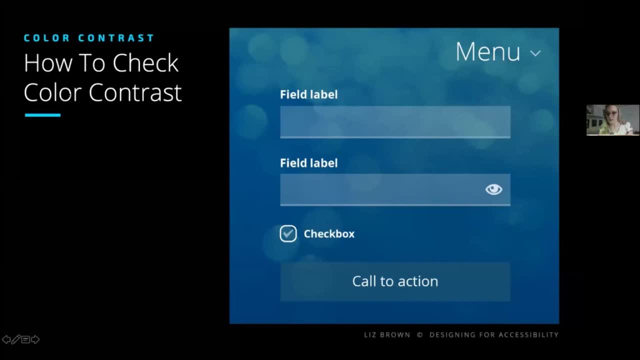 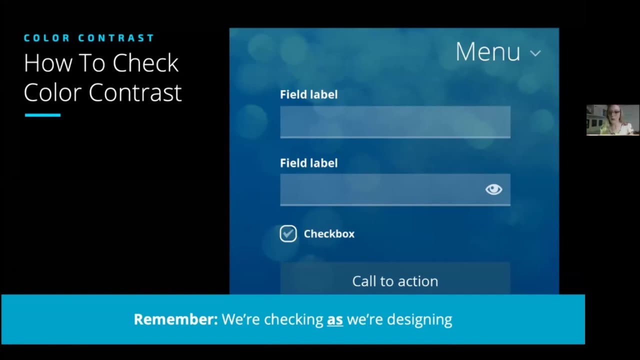 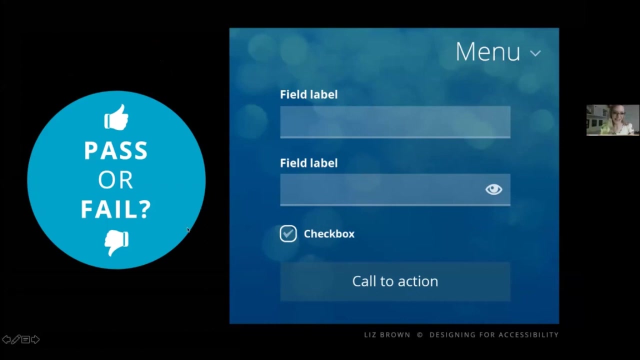 ratio for your information. bearing elements. Okay, let's go back to this here And also remember we want to be checking for color contrast as we're designing, We don't want to do it afterwards. So now, what do we think? Pass or fail? Did anybody's answer change? Thumbs up or thumbs? 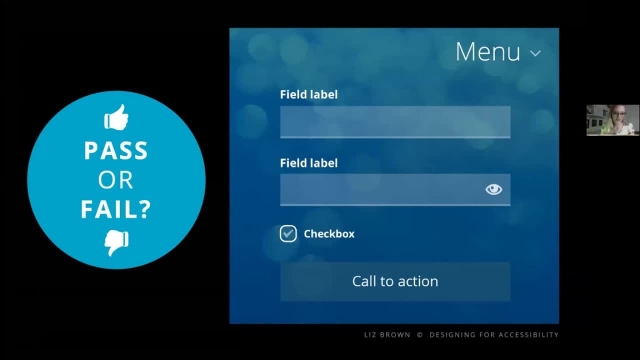 down. Is it a pass or a fail? Well, if you said fail the first time, you were right. So let's just go through these things one by one. So let's go through these things one by one, And then we're going to. 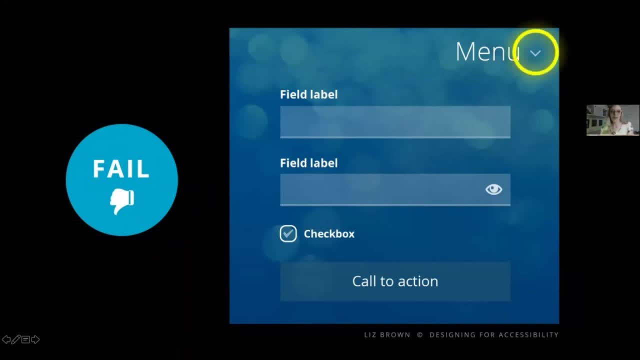 go through these things one by one. So let's just go through these things one by one And then we're going to really quick. This little carrot icon at the top- is that information bearing? Yes, because if you didn't see it, 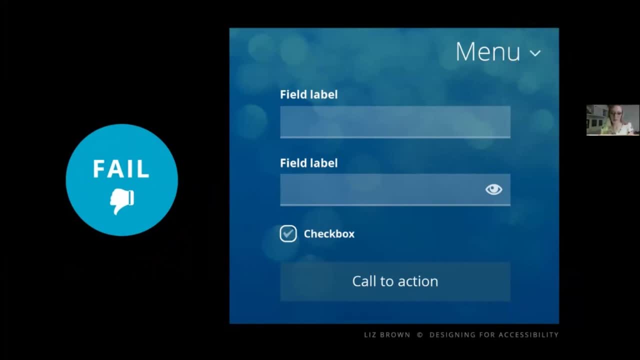 you wouldn't know that there's drop-down functionality. So we make that. have ample contrast. This little underline for the field input: is that information bearing? Well, you wouldn't know where to type your input if you couldn't see that underline. So, yes, that's information bearing. We need to make that have. 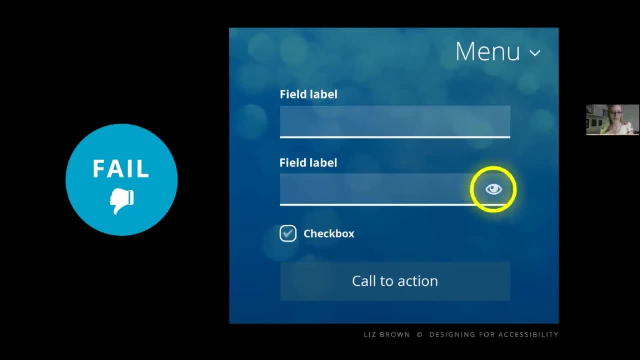 ample contrast. How about the little eyeball icon? That's a standalone icon. There's no little text label next to it, So that's a standalone icon. That's a standalone icon. There's no little text label next to it That says toggle visibility or anything like that, So it's information bearing. We need to make that have. 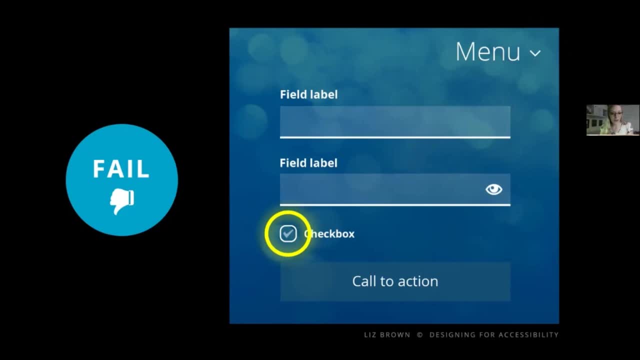 ample contrast too. The little tick mark in the checkbox. that tick mark is conveying that this checkbox is in its checked state, And states need to be compliant with contrast as well. So we fix that. And then the last one, the button. That one's just. it kind of looks like plain text, right It's. 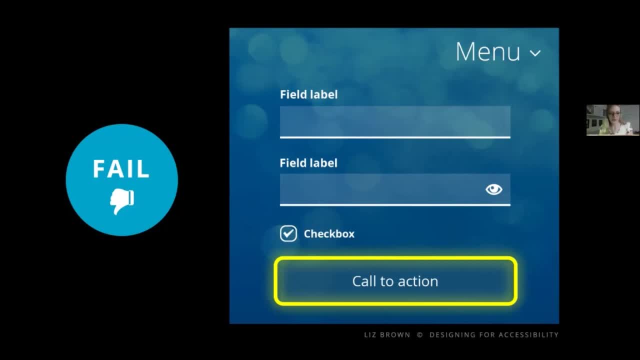 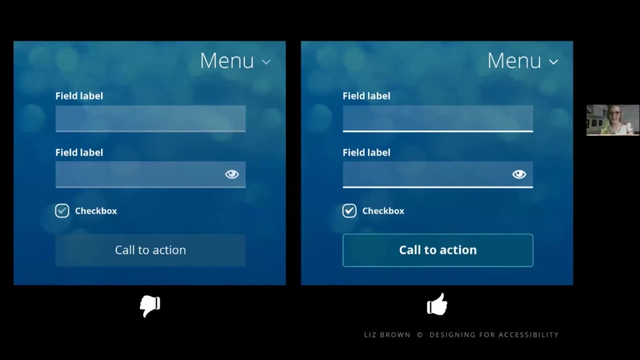 not doing really well for accessibility or usability. The signifiers aren't really giving us that perceived affordance of a button, So we fix that as well. And now this is much better and it passes All right. So there's our before and after, And now that's the end of strategy number one. 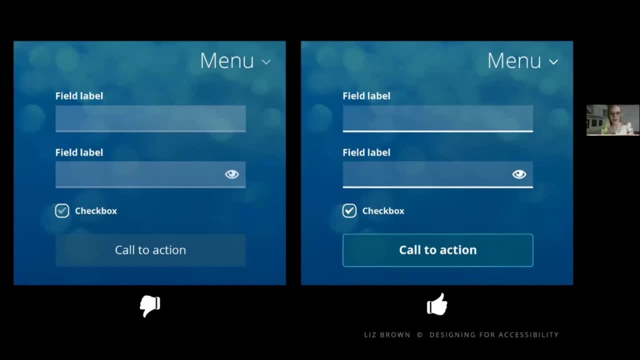 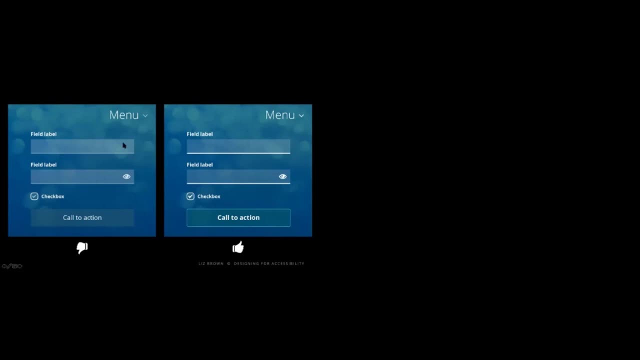 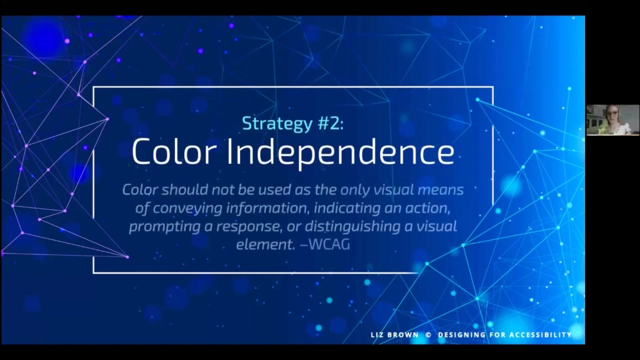 So any quick questions before we move on to strategy number two. Okay, Let's really. let's sail on over to strategy number two. So number two, this is color independence. So, starting with a simple definition for an interface to be accessible, color should not be used as the only visual means of. 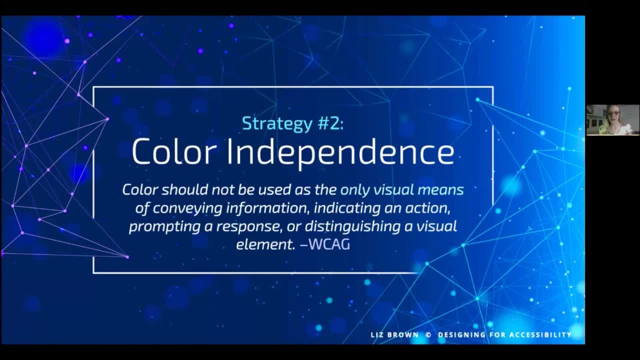 conveying information, indicating an action, prompting a response or distinguishing a visual element. So to say that more simply, we can't depend on color to communicate information, like red to communicate that something's offline or green to communicate that something is online. 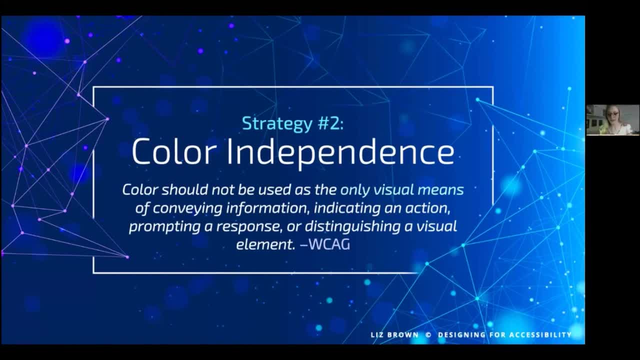 If we rely on color alone, that's called color dependency, where users are dependent on being able to see the information. So if we rely on color alone, that's called color dependency. We want to be a color to understand something And we want to be color independent. 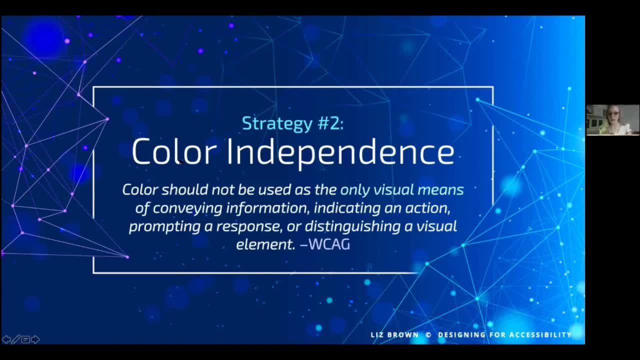 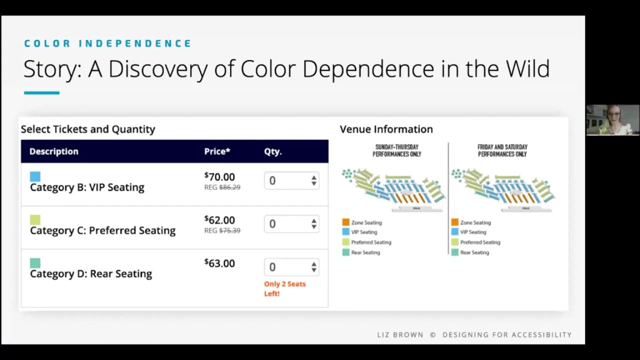 So not dependent, but independent. It's also important to note that this should not discourage color coding. So still use color, just not as the sole means of visually conveying something meaningful. I have a little story for you. So my sister got engaged right before the pandemic. 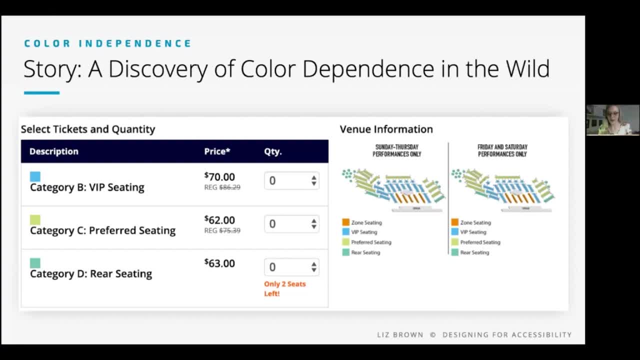 And as her maid of honor, it was my job to plan the bachelorette party, which I then turned around and canceled everything because COVID hit. But before that I was on this website and I was checking out various show tickets, like Cirque du Soleil. 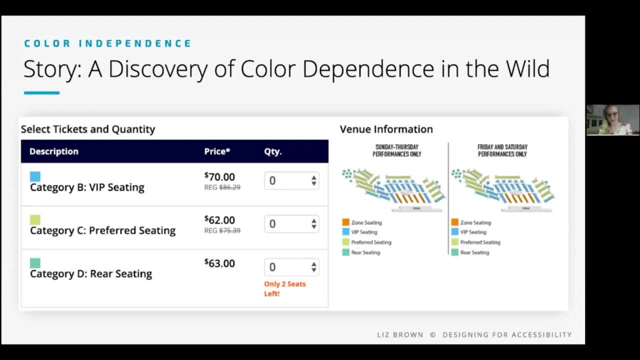 and stuff like that, And I noticed a terrible color dependence issue. Can you see it? So I'll point it out to you. So this website is showing that blue means VIP seating And then we go over here to the legend And okay, blue means VIP seating. Now we go look at the. 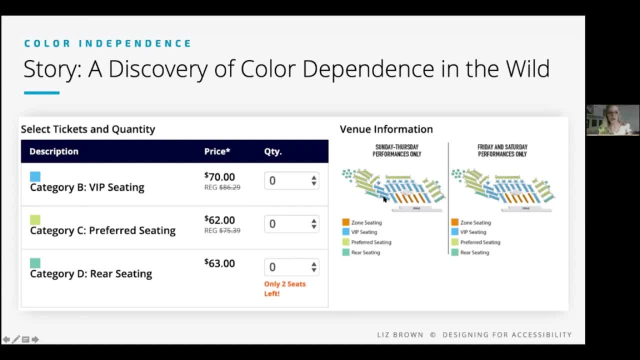 the seating map of the venue and which one's blue. If I was completely colorblind- and I could, I only saw the world in grayscale- I would have no idea which one was blue. Or if I was colorblind in the sense that I got colors mixed up and I got blue and green mixed up, or I got blue and 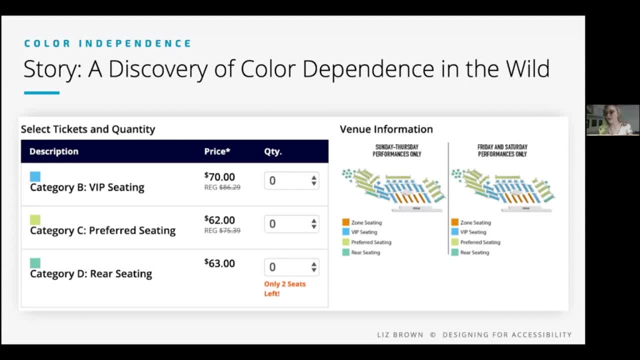 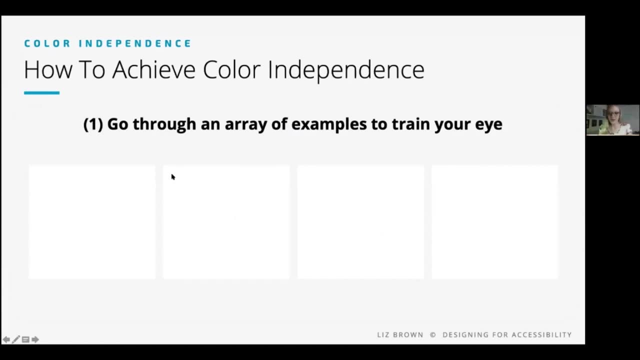 orange mixed up, I'd be buying the wrong seats, right? So that's a huge color dependency example And that makes that makes for really bad user experience, right? So how do we achieve color independence? Number one: learn how to recognize color. 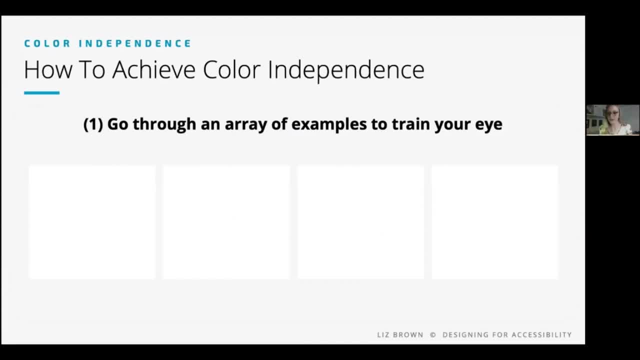 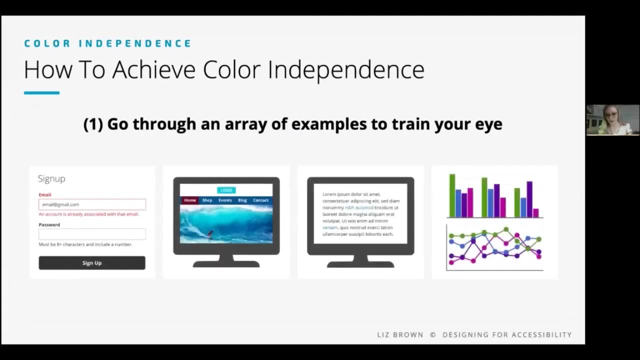 dependence by going through an array of examples to train your eyes to recognize it. And then the number two thing that we do is we test for color dependence by using the grayscale test. So take a look at these examples down here, starting with the left, and watch what happens. 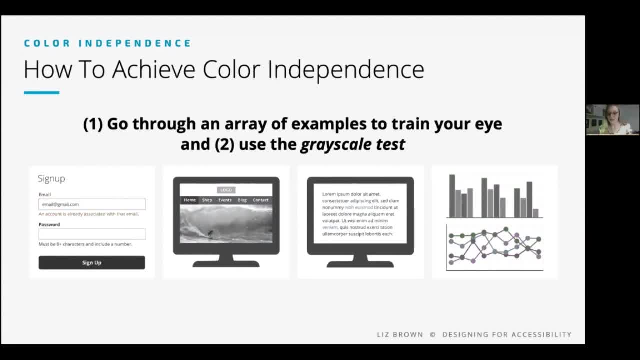 This is the grayscale test. We just turn the design grayscale And then we ask ourselves or somebody else with fresh eyes, now that the hues are gone, is there anything that I can no longer one identify or two tell the difference between? So let's go through some of these examples right now and see how we do. 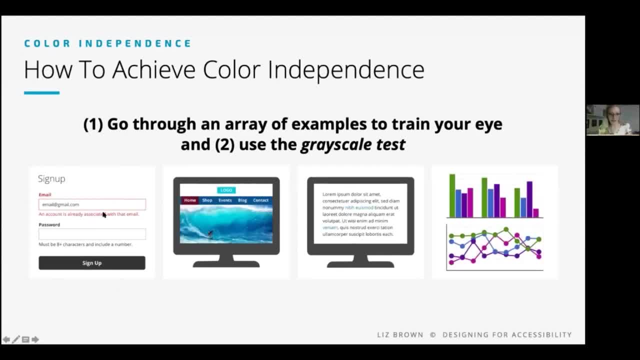 So this first one, this is showing an error message, right, And we know it's an error message because it's got that red error text and the red field border. Well, when I turn a grayscale can you tell there's an error? 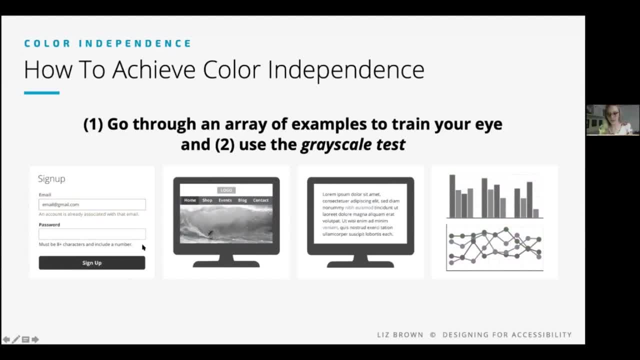 Probably not, because now that error text looks just like the helper text that we're seeing in below the second field. Okay, next example, this second one- we can tell from the main navigation that we are on the home page because that's highlighted, and then the other main navigation items are navy, blue and home is. 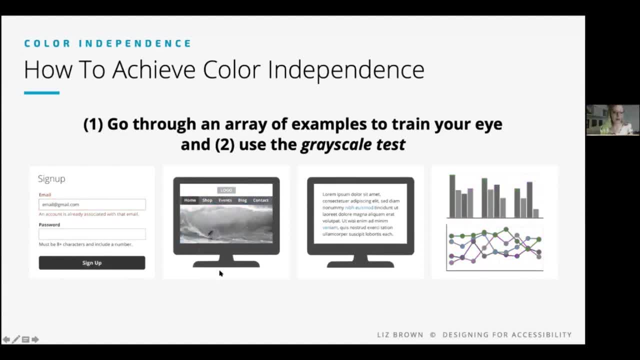 maroon. Let's turn it grayscale. Can we still tell what page we're on? Not so much, right? It kind of all looks like gray and gray and gray. Okay, let's look at the third one. there are some text links in here and they're turquoise. And we know that they're links because 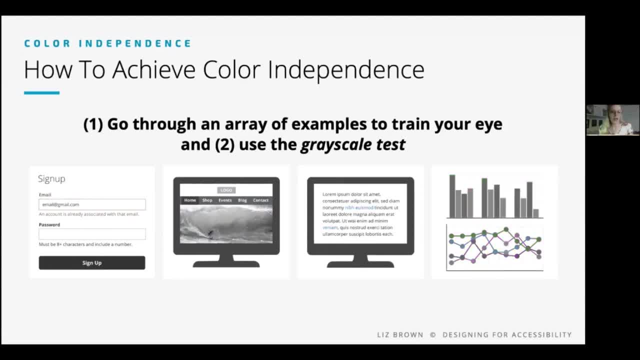 they're turquoise. We turn it gray scale and now the links disappear. So you wouldn't those links completely blend in with the other text because the designer didn't underline their links that had surrounding text. So always underline your links with surrounding text. And then, lastly, for 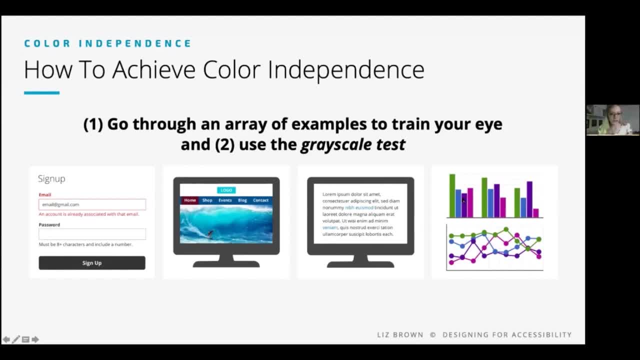 any sort of data visualizations. if we had a legend and the legend said: green is the United States, blue is Canada, purple is Mexico, well, if you're colorblind, all of that means nothing to you, because you can't see that. So those are some examples, And remember, we're checking for. 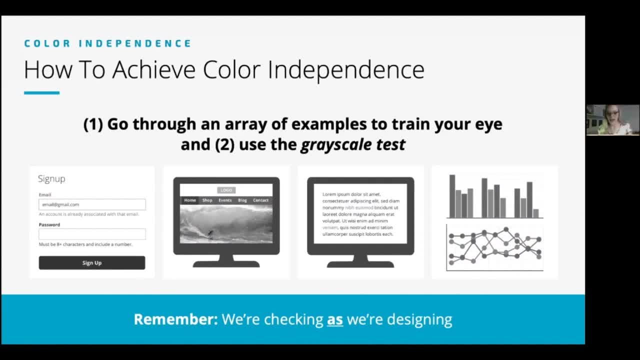 color dependence. We're checking for all this accessibility stuff as we're designing. Just like we don't add usability at the end, we also don't add accessibility at the end. Okay, so there's three steps to achieving this strategy. We're going to 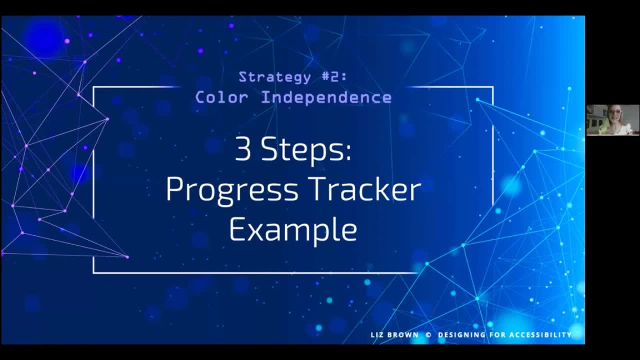 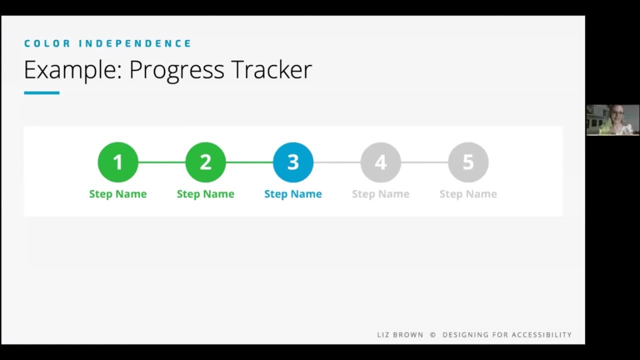 design a color independent progress tracker as an example to take us through these three steps. This is going to be fun. I love designing progress trackers. Okay, so take a look at this progress tracker right here. This is what we have so far. So, in regards to color independence, 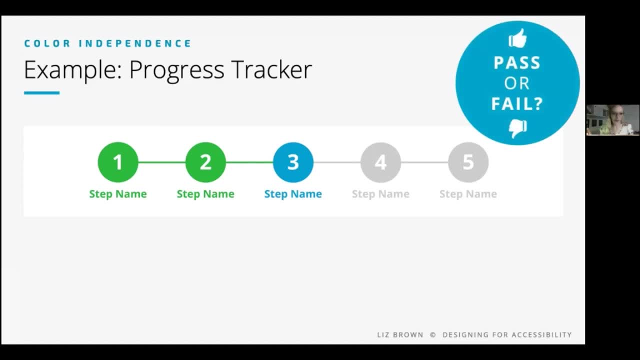 does this pass or fail, And you guys are probably getting a hang of this now. but just give me a thumbs up or a thumbs down to the camera. Thumbs up meaning it passes- color independence. thumbs down mean it means it fails. color independence. 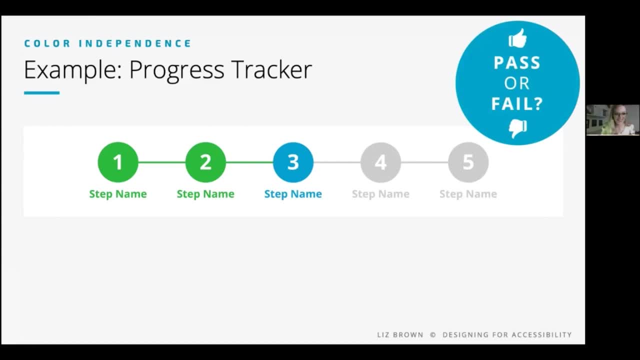 Okay, good, I'm seeing some thumbs- Awesome. Yep, you guys are getting a hang of this. I'll show you it in grayscale, because that's the first thing we should do anyways. So we check in grayscale and, yep, it fails, because now the green and the turquoise look exactly the same. So we don't know. 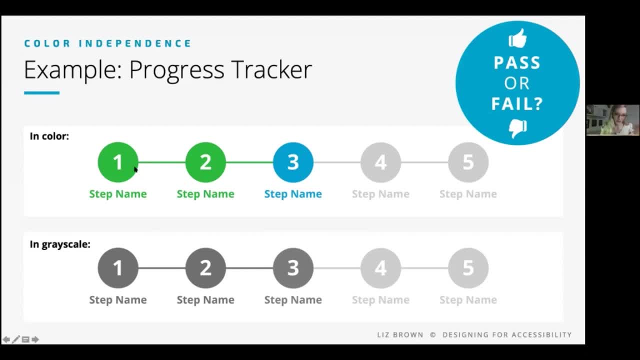 So step one and two, we have successfully completed those in our little fictitious example here. So those are done. Turquoise is the current step and gray is the future step. So if we can't differentiate those three states in grayscale, then that's a color and that's a color dependence issue. 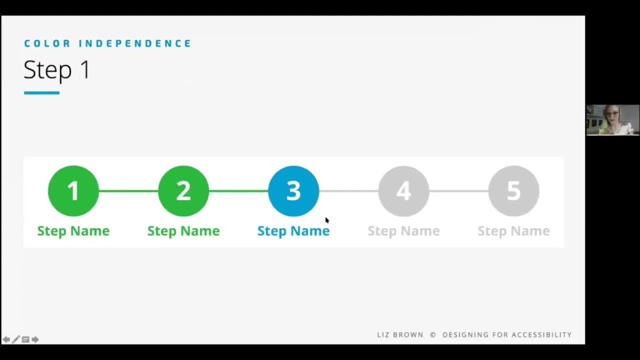 So let's fix it. Yes, like I said, that's a fail. So first to fix this. what's step number one? Step number one: we're going to turn the whole thing one color, like all black or all graphite. 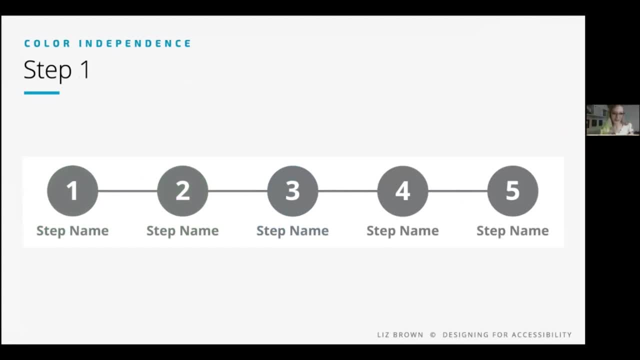 gray, And this is going to probably remind you of wireframing. you know, when we work in black and white, If you're putting in shades of gray, that means you're trying to communicate stuff with with color and you're interjecting color dependence. So turn it all one color. 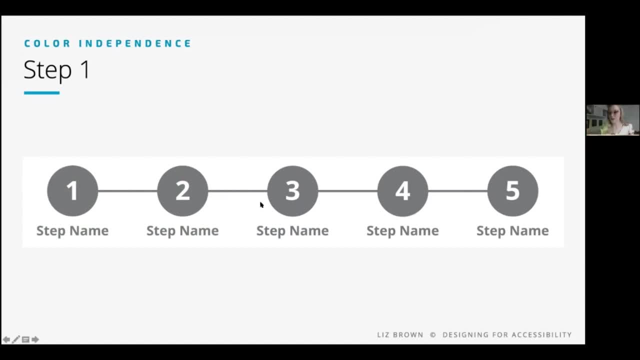 And now let's start differentiating our three states. So the steps you've successfully completed, the step you're currently on and the future step. So those are three states: past, current and future. So let's differentiate those using structural elements only. 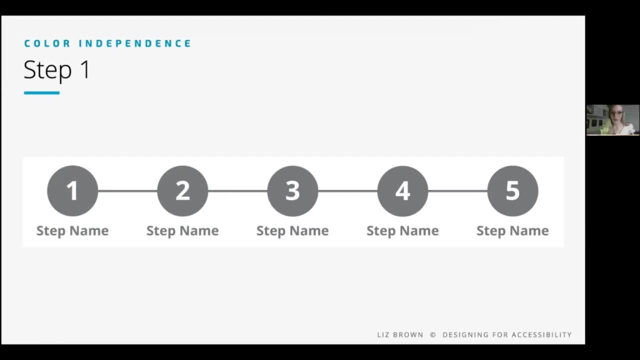 So what's? what's a way that we can differentiate them without using color at all? So how can we do this? Well, let's see, We can't use color right, So we need to do it structurally. How about hollow versus solid? So let's do that for step two. Okay, so now my future steps are: 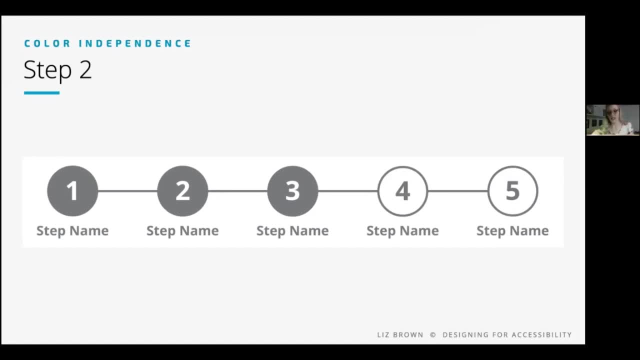 hollow, But now we still need to differentiate between the past steps and the current steps. So how could we do that? We've already used hollow versus solid. How about using some icons? So, step three: let's throw in some icons. That'll be for number one and number two. I'll 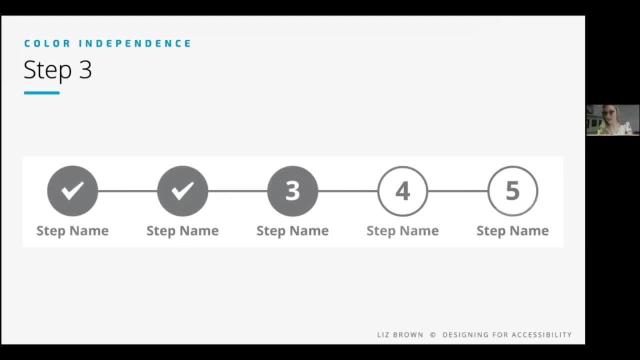 flip between those so you can see what I did on number one and number two. It's only a five-step progress tracker, so it's okay if you can't see the numbers for those steps you've already completed. All right, so now we have successfully differentiated all three states. 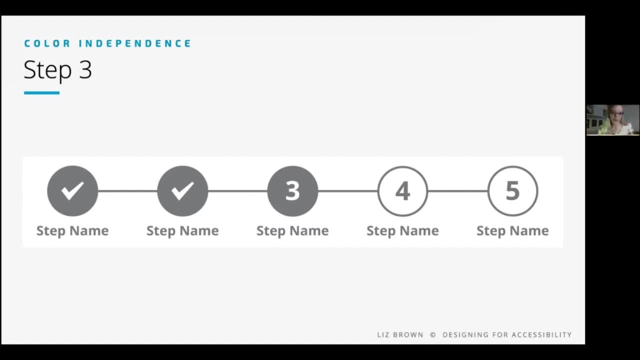 without using color at all, And we can stop here if we want to. This is now accessible, But we could take it even further and we're trying to be really good designers, right? So let's see what else we can do to like further enhance this structurally. So enhancement. 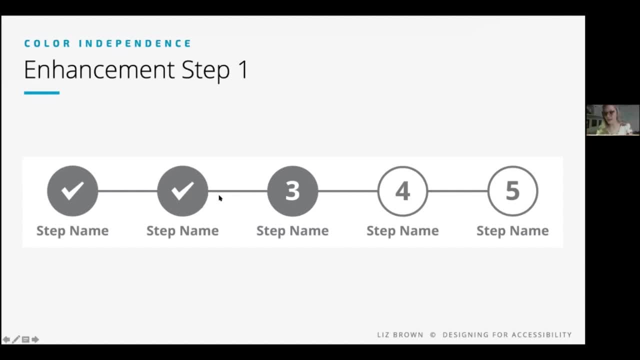 of our text. So here we can see that we've just changed the font and the font size. So we've changed the font size And we can see that it's a little bit thicker. that's why I made this step thicker, And then we can also play with the thickness of this connector. 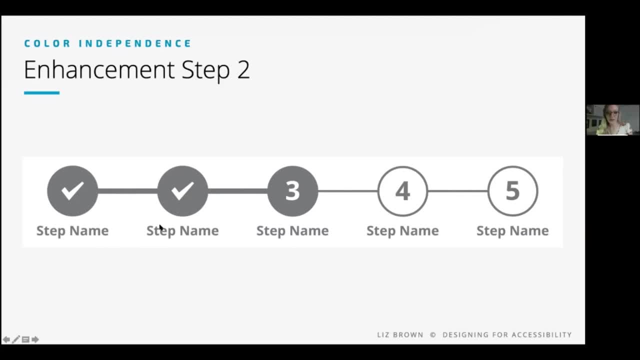 line. So here I made the it thicker between the past steps leading up to the current step. What else could we do? We could also play with the text formatting. So the step names down here. we could do bold, italic, so on. So I'm going to make the current step extra bold, so it really 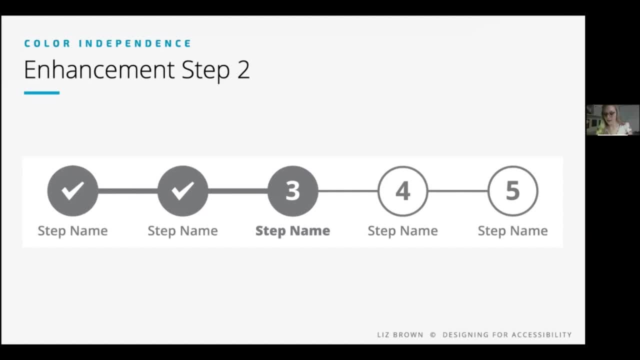 The other thing that I want to do, that I want to make visually clear about this progress tracker, is that you can click any of these steps to bounce around, So these are all clickable. How do you visually show that these are clickable? I thought of a whole bunch of fancy ways I could do it, but at the end of the day, it's actually the simplest solution. that's the most clear. 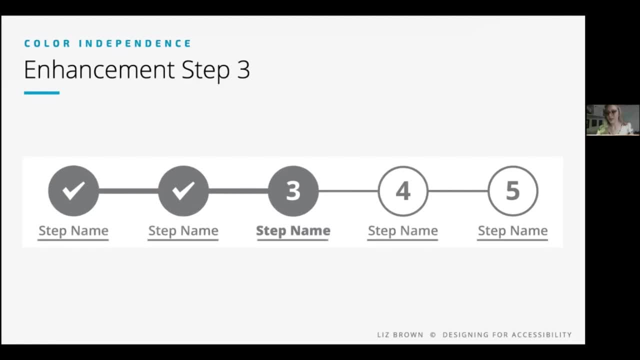 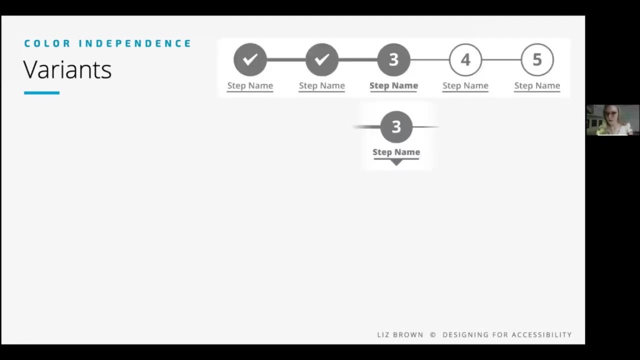 And that is to just underline the steps, And now that's undeniably clear that you can click on these to jump to any page in the workflow. So there's a lot of other structural things we can do to differentiate our three steps. These are just some examples, Right? So, for example, we could also, for the current state, we could pull a triangle down here. 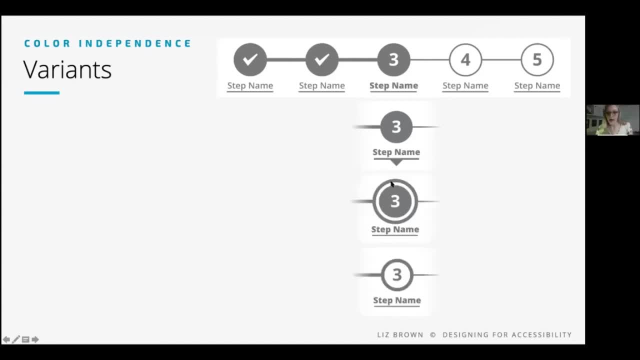 We could put another ring around the three. We could make the current state hollow but make the stroke around it thicker to differentiate it From these future steps. four and five that are have a thinner stroke And, speaking about those future steps, we could make them a dotted line instead. 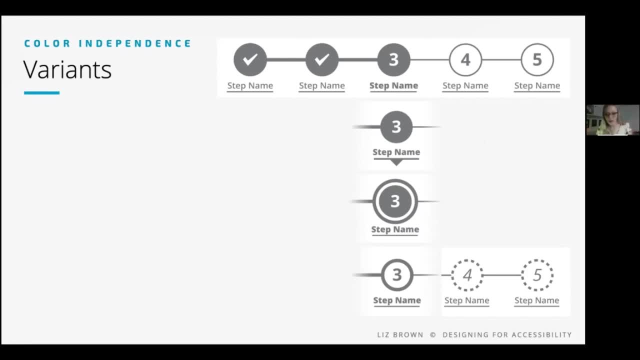 So there's a whole bunch of stuff that we could do here structurally to differentiate these OK. so once we have it, however, we want the last thing to do is give it a paint job, And that's important to still use color, because it helps people who can see color. 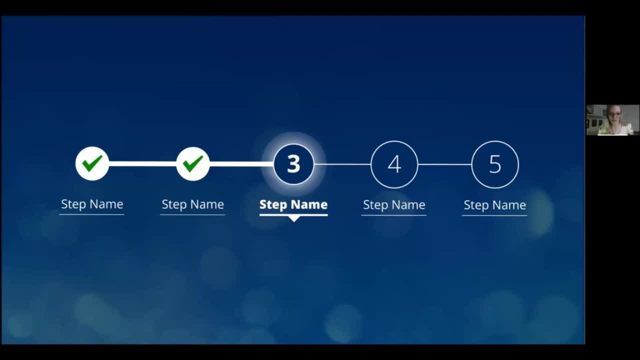 So we style it up with color. however, it matches the color. That's the branding we're going for. So I added in green for the check marks, I added in this decorative aura around number three, And so now this is accessible and color independent and we're all done. 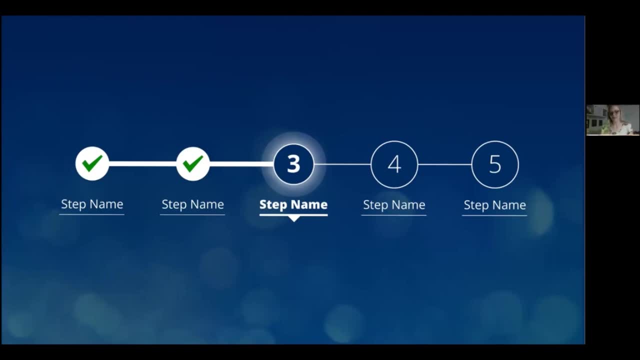 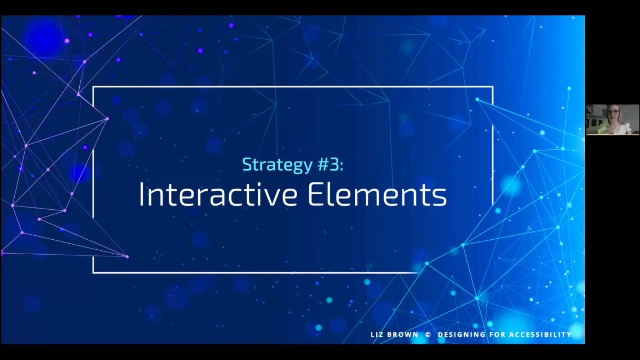 So that's how you design for color independence. All right, Any questions? All right, Let's get on to our last strategy. This one's going to be a quick one to share. Strategy number three is about interactive elements Like buttons, links, clickable icons, radio buttons, checkboxes, accordions, clickable cards or tiles, and so on. 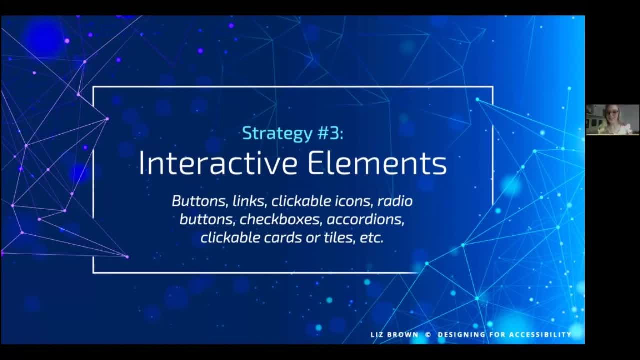 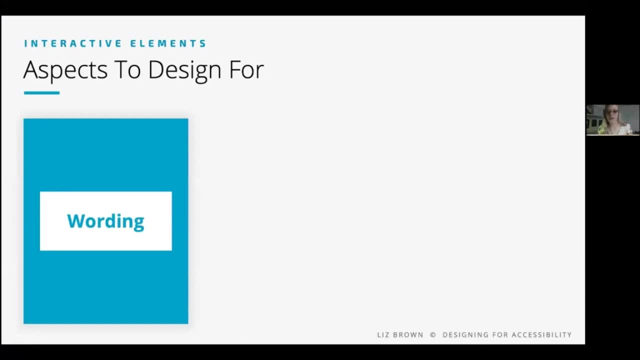 So there is a lot that I could share when it comes to designing accessible interactive elements. For example, we could talk about wording like: do our interactive elements read like they're interactive? Are we using tasks to specific words? Do we lead with the action words? 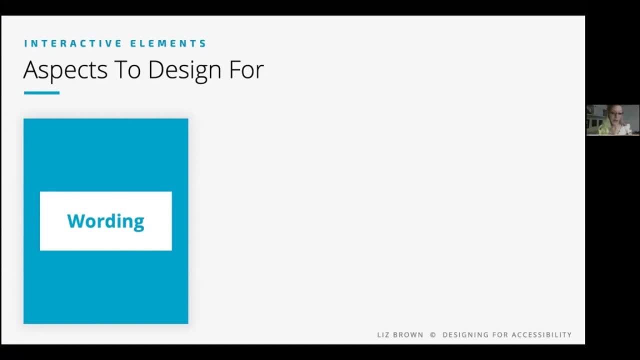 Is each button or link label unique from the others? Are they unique from the others? on the page, We could talk about styling. So are the interactive elements styled to look interactive? So, talking about shape, shadows, label capitalization, proximity, size, all of that good stuff. 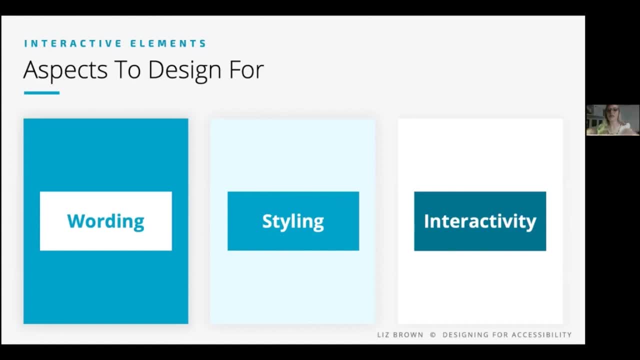 And then there's also interactivity. So do our interactive elements respond like they're interactive? So that's talking about interactive states like hovered, focused, selected, toggled, active, all of that. So a lot of these Sound like just good usability, don't they? 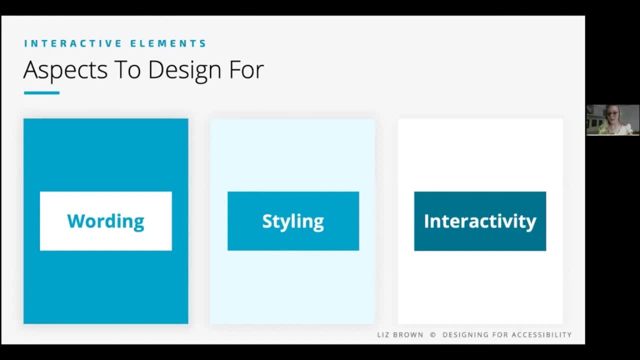 Well, like I said, accessibility is usability for all, And when you have a disability- temporary, situational or permanent- all usability issues are exacerbated. So to have an accessible website is to also have top notch usability. Out of all of these aspects to design for when designing accessible interactive elements, I picked just one thing to share with you guys. 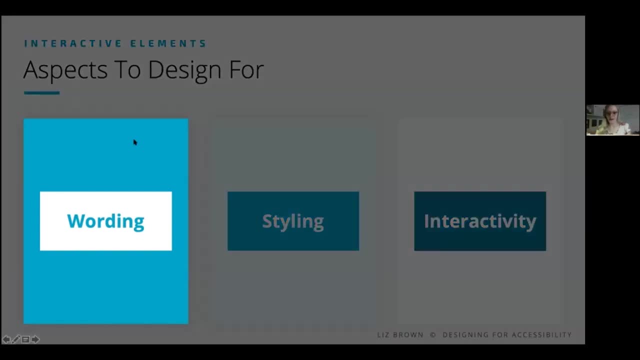 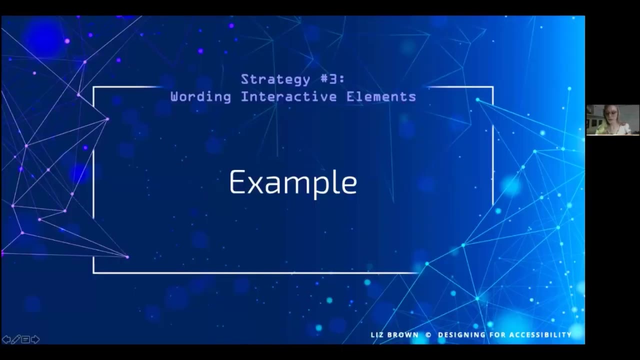 And this one thing is in regards to wording. So let's take a look. When I was first learning about advanced accessibility, this is one of the design problems that was the most difficult for me to find an accessible solution for, And, of course, after I did figure out a solution, it seemed obvious. 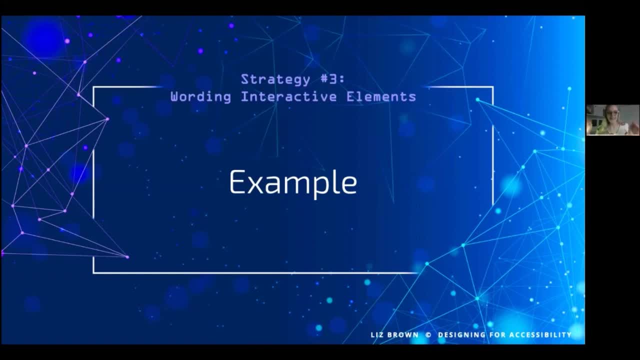 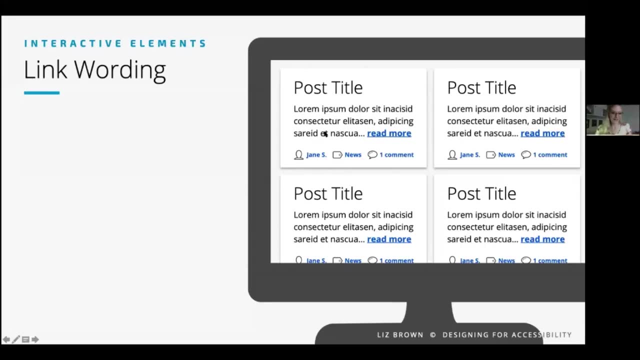 But, man, I really had to work for it. So I hope that my blood, sweat and tears saves you some blood, sweat and tears. But let me pose the design problem to you, And maybe you already know the answer to it, Who knows? 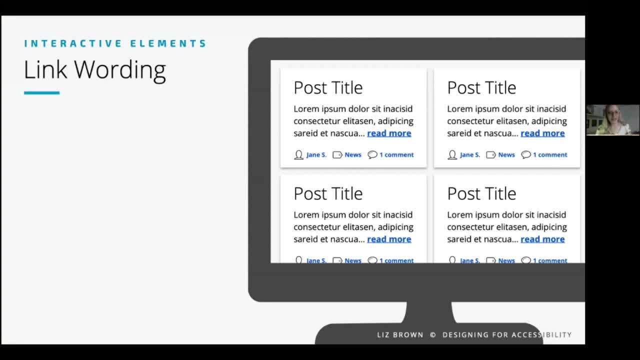 All right In regards to link wording. do you see any accessibility or usability issues with the links in this little mockup? So take a minute and just think about it to yourself. What could it be? What's wrong with these links? Okay, 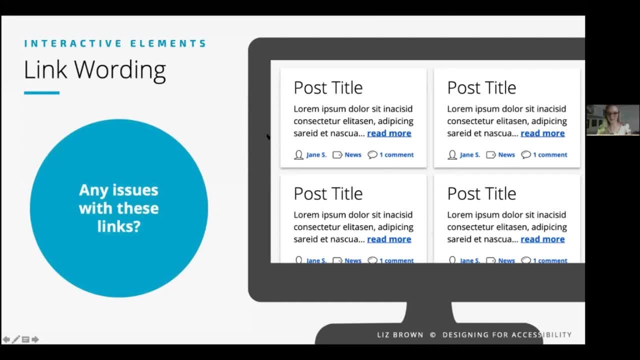 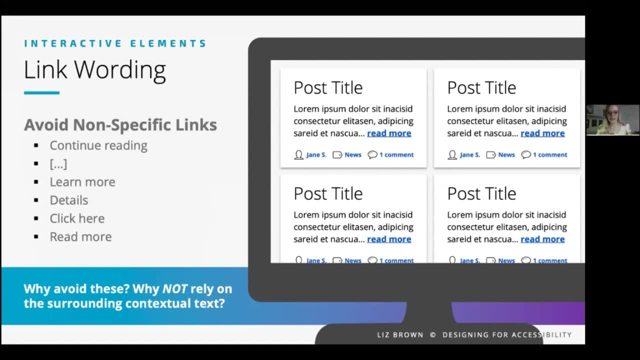 I'm going to give you a hint When it comes to link wording. we want to avoid nonspecific links like continue reading, dot dot dot. learn more details, click here. So do you see the issue now? It's all those repeated read more links. 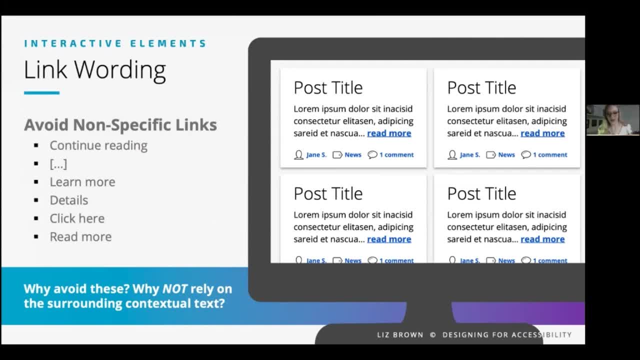 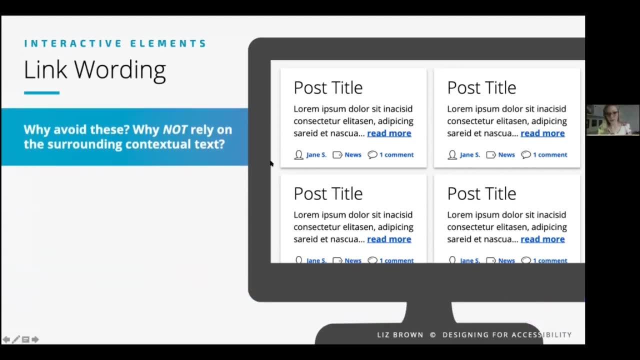 But why is it so important that we avoid them? Why do we not want to rely on the surrounding text to give you context as to what you're reading more about? Well, it's for three main reasons. Let my PowerPoint catch up here. 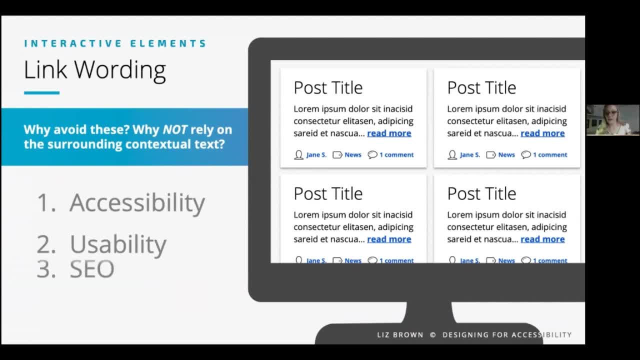 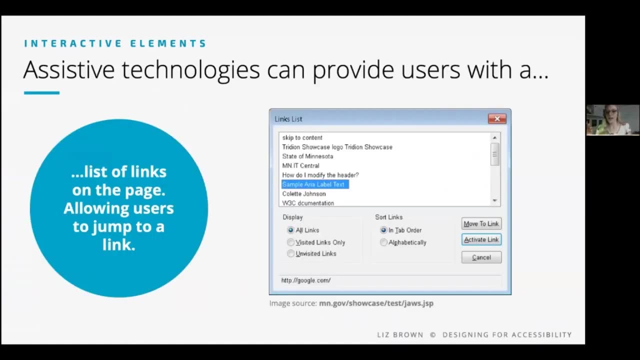 So for three reasons: Nonspecific links. they decrease the accessibility, They also decrease the overall usability And they negatively impact the search engine performance. So how findable the content is, Let's talk about the accessibility aspect. So, let's talk about the accessibility aspect. 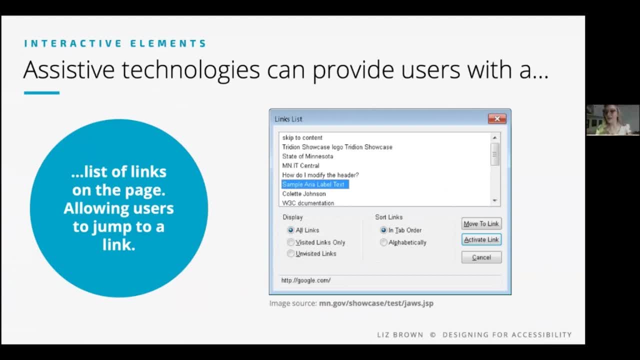 So let's talk about the accessibility aspect. So assistive technologies like screen readers. they can provide us with a list of links on the page that then allow the screen reader user to jump to a link. So, for example, say you're blind and you're navigating a website. 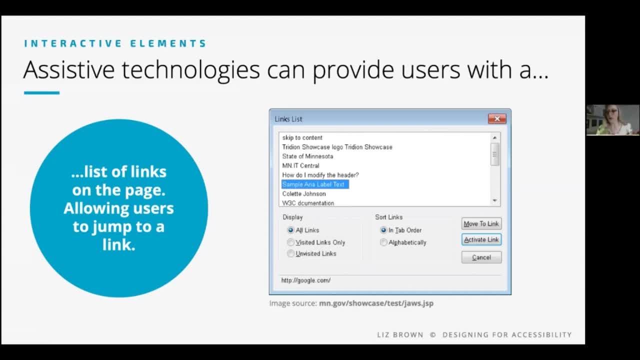 You click a keyboard shortcut on your keyboard to bring up this pop-up. This is a feature of your screen reader And this pop-up shows all of the links on the page And the screen reader reads them out loud So it says: skip to content. 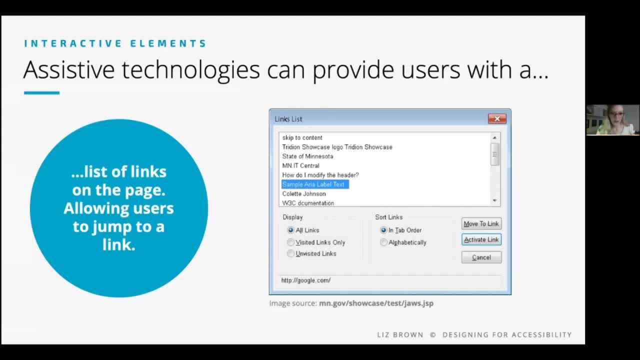 Try to showcase logo, Try to showcase State of Minnesota. How do I modify the header, And so on. So when you, as a user, hear one of these links that sounds like a place you want to go like, okay, that's the page I want to go to, or that's the link I want to click on. you select it and the screen reader jumps you to that page of the interface. 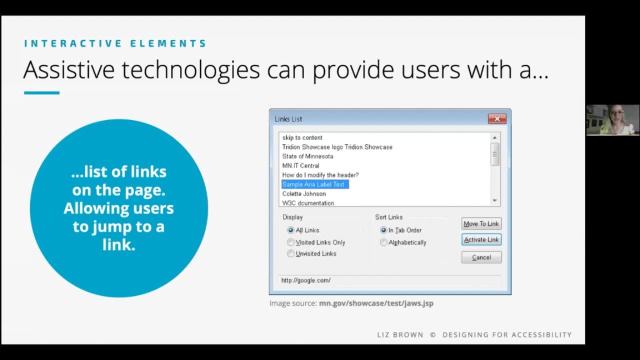 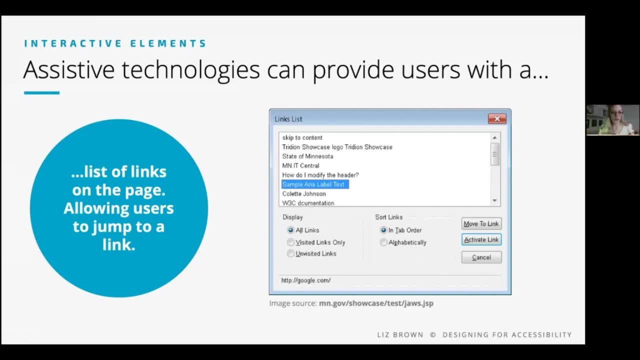 And it's bad for usability, because people who visually scan a page- usability studies have shown that we often when we're skimming a page, we're reading just the links, just the clickable stuff, And so when you're visually scanning a page, same sort of functionality as what the screen reader is duplicating over here. 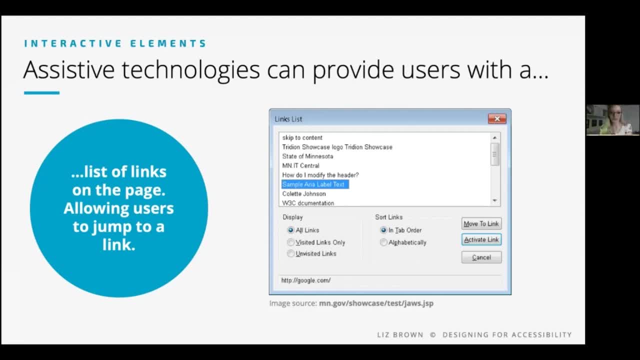 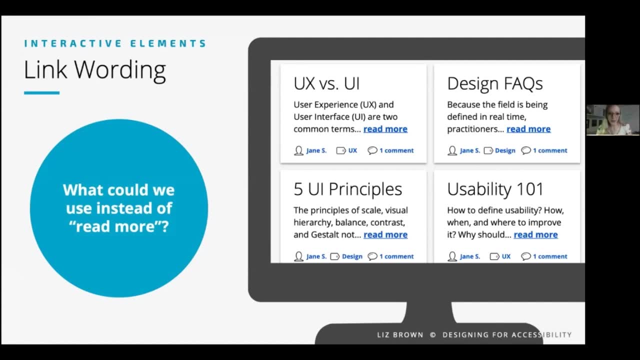 You don't want to just read, read more, read more, read more, because it's not very helpful. So what could we use instead of the read more links? So I was thinking about this and I was like, okay, maybe I could say read full post, or just full post, or go to article. 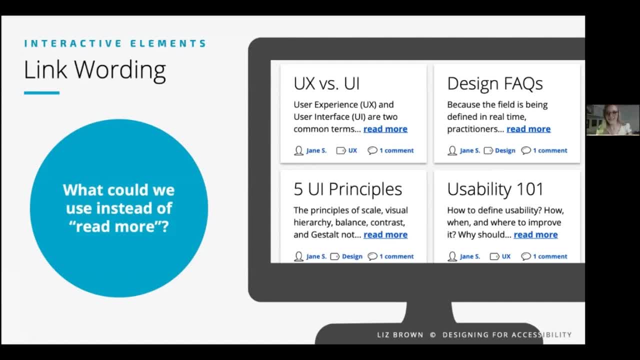 But all of those have the same issue right, Like they're all nonspecific duplicated links. So how do we solve for this? Do you guys want the answer? This took me way longer than it should have to figure out, Okay, So as I started to learn more about how to write really optimal links and button text, it became clear that what we really need to do is be explicit about where that link or button is transporting you to, or what action is it triggering. 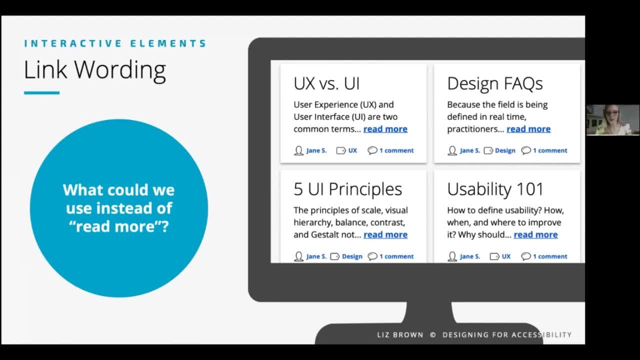 So transparent about the transport or the trigger. So what page is that link going to? Well, for this first post in the top corner, it's going to a page that's titled UX versus UI. That's the name of the article, So that's what my link should say. 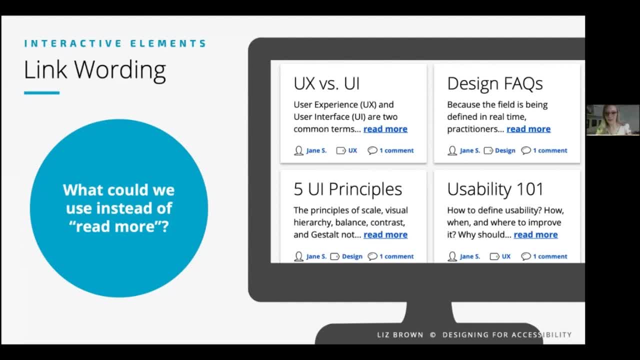 That way, my link is being transparent about where it's taking you. You're going to a page that's about UX versus UI, So I could add that to the link and it would say: read more about UX versus UI. But that's going to be a very long wordy link, right? 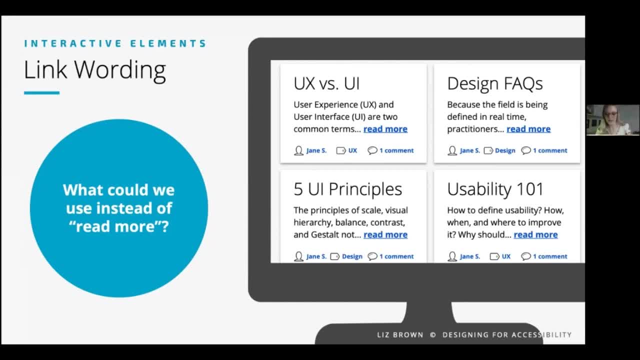 Especially if I have article titles that are like entire sentences. So that wouldn't really be the most elegant or flexible solution. So what could we do instead? Well, I already have the words UX versus UI there at the top in the title. So the simplest solution is drum roll to just link that title right there. 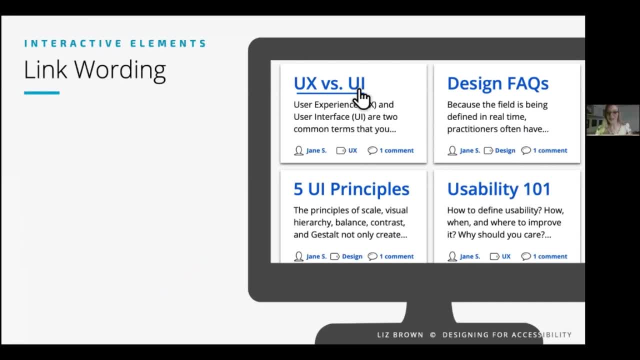 And then you style it to look clickable, so people know. So there you go Now the list of links that the screen reader pops up. it will now read all the post titles for each of these, instead of saying, oh, I'm going to do this. 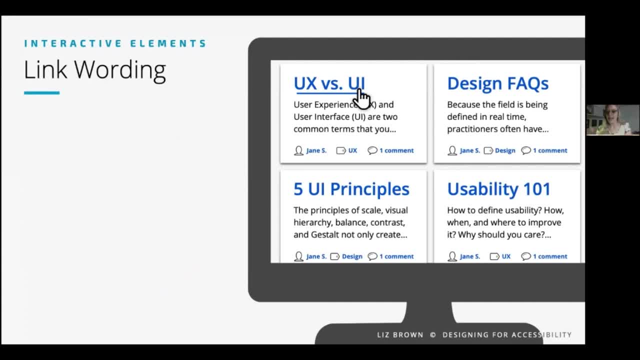 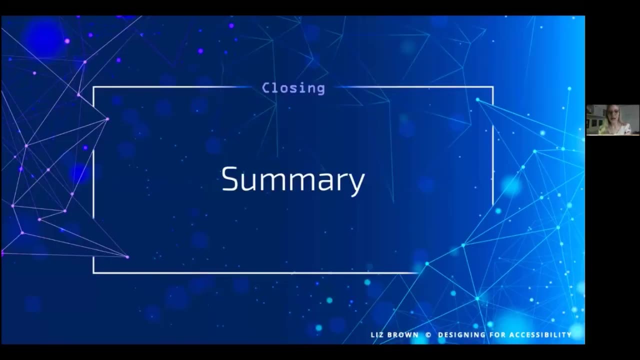 Instead of saying: read more repeatedly Now. this is so much better for accessibility, usability and SEO. Okay, So that's the end of strategy number three about wording interactive elements. Allow me to summarize everything we've talked about here for you. 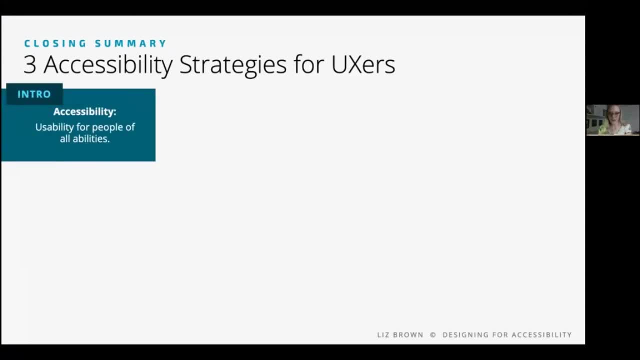 So our three accessibility strategies. First, we started with an intro And we talked about how accessibility is for people of all abilities And how disabilities can be temporary, situational or permanent. We talked about WCAG, how that's like the golden list of guidelines to follow. 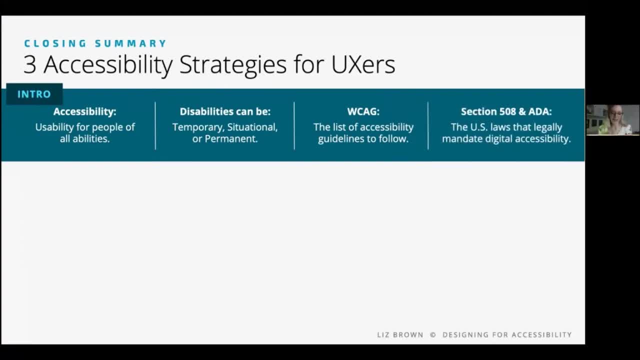 And then we talked about Section 508 and ADA. So those are the US laws that legally mandate digital accessibility. Then getting into our strategies: strategy number one that's for color contrast And that helps people with low vision. So information-bearing elements. 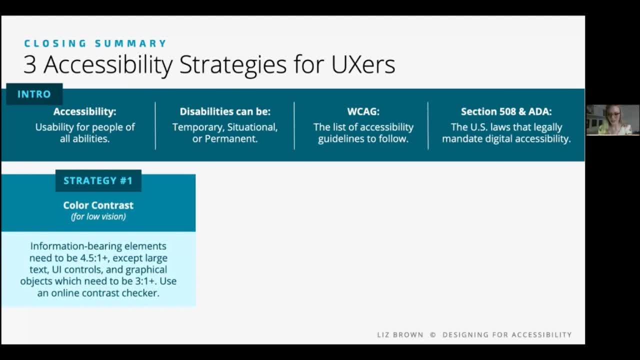 They need to be that four and a half to one contrast ratio, Except large elements, UI controls and graphical objects. Those need to be three to one or greater, So you can use a contrast checker, an online contrast checker, to test those out. 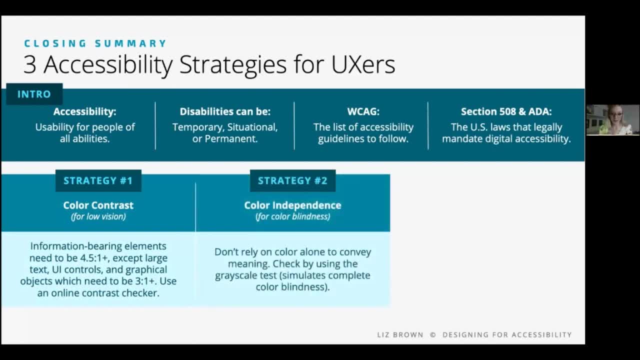 And then strategy number two that was about color independence And that helps people that have color blindness. So the strategy is to not rely on color alone to convey meaning. So check for color, Check for it. Check for it by using the grayscale test, which simulates complete color blindness. 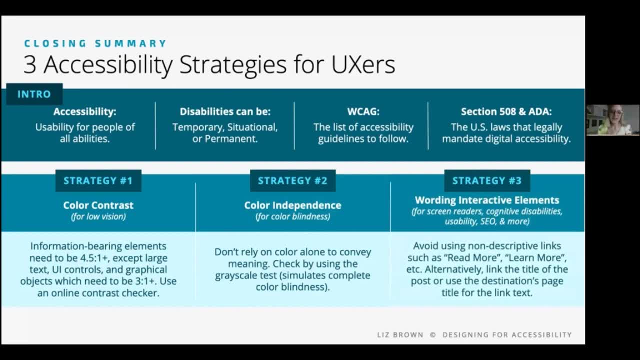 And then our last strategy, number three. that's about wording interactive elements, So that helps people who are using screen readers, people with cognitive disabilities, And it's also just good in general for usability plus SEO and other things. So that strategy was about avoiding using nondescriptive links such as read more, learn more, continue reading. 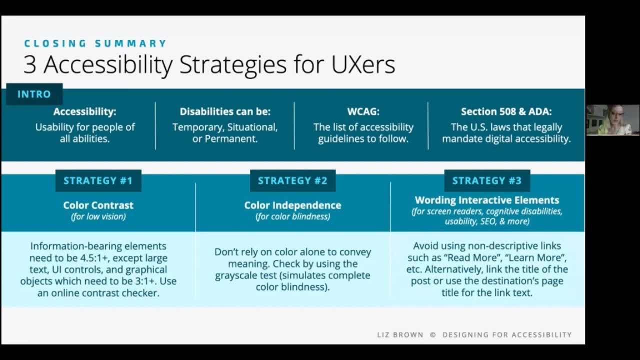 And alternatively link the title of the post Or use the destination's page title Or the link text. And remember, with all of these accessibility strategies, we need to check for these things as we're designing, not afterwards, Because, like I said, we don't add usability at the end. 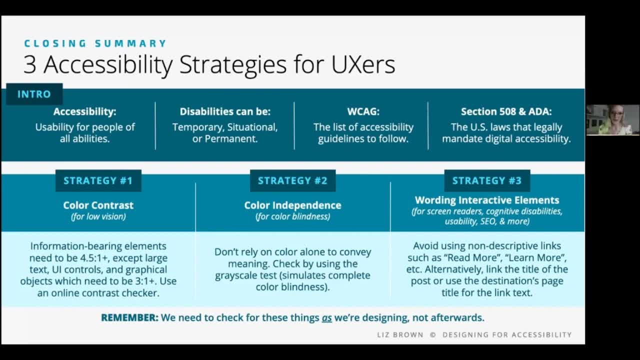 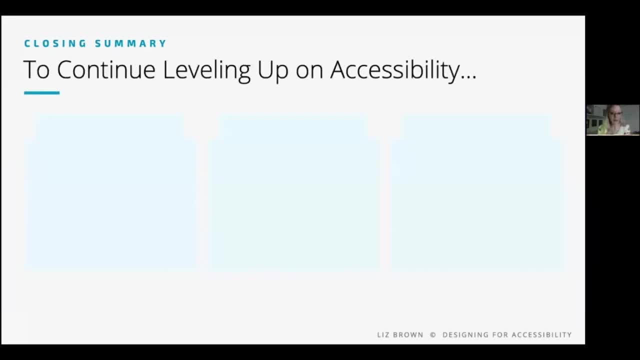 We can't be adding accessibility at the end either. It just doesn't come out as good, right, Okay. So if you want to continue leveling up your knowledge about accessibility, I have a couple things to share with you. I'll post these in the chat here in a minute. 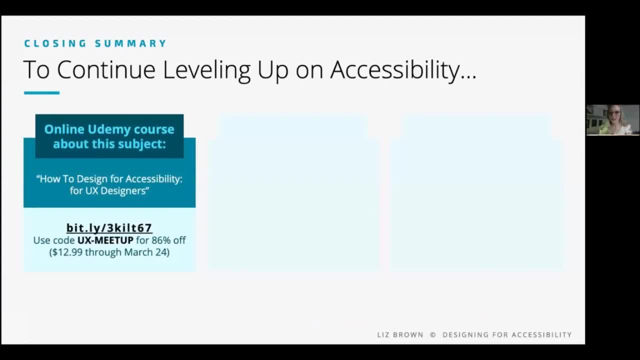 But, like Ben mentioned, I have a course that I just recently launched about this topic. It's called How to Design for Accessibility And it's specifically for UX designers- Just the stuff that you need to know as a designer. We don't like get into the code. 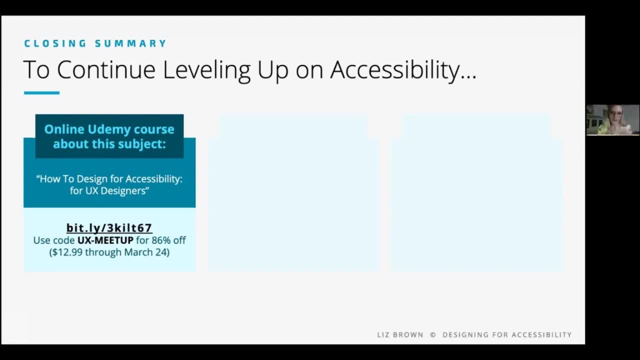 So there's a link to the course if you want to check it out- No obligations, obviously- And there's a coupon code that Udemy allows me to give out to my friends, family associates, colleagues. So I'm giving you guys my best one. 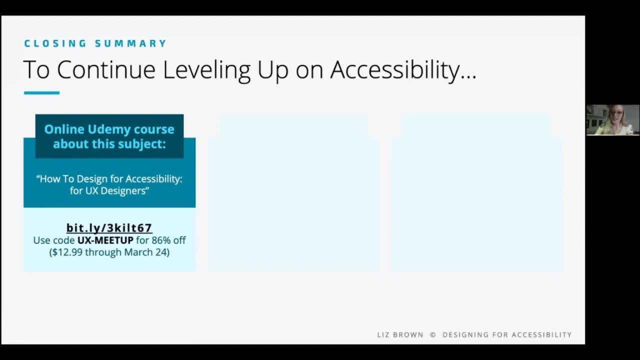 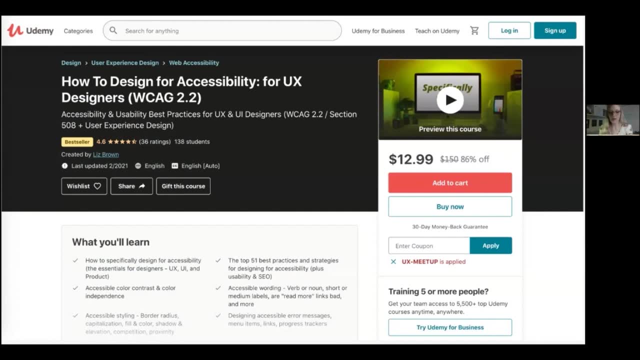 It is 86% off. So if you go to that link there, it brings up or it goes to a page right here And there's a video in the top corner. You see, there's a video And that's just a couple minutes long. 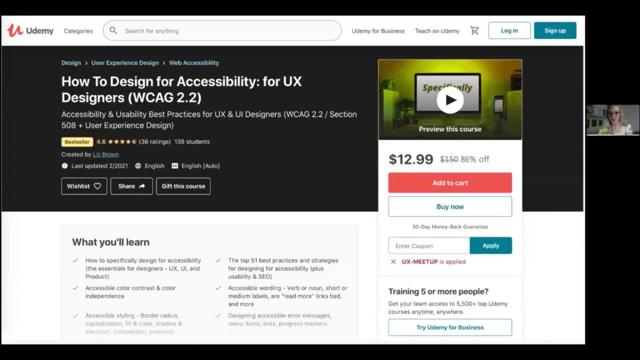 And it previews what the course is about. So just want you to know that you can check that out before committing or anything. Something cool is that after completing this course you'll get a really nice certificate And then you can go post that to your LinkedIn, like in your feed or on your profile. 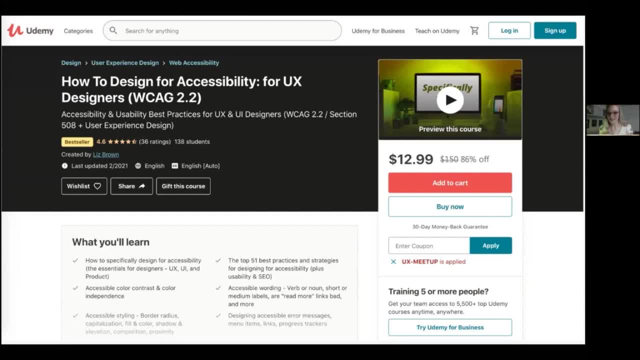 And it's fun because it's like your professional bragging rights to show that you're trained as an accessible designer, So I love that. I've seen people do it. I'm like, oh, I want to do that with all my Udemy courses too. 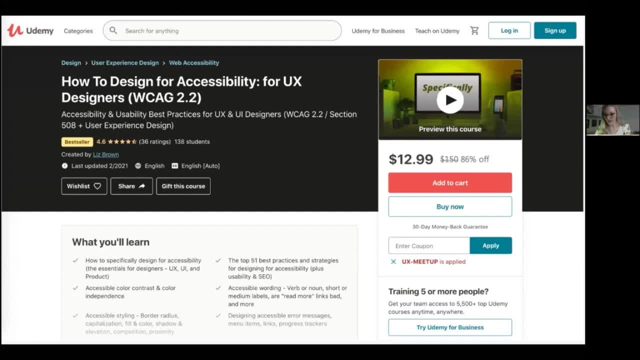 So I launched this just like a month and a half ago, And I've been so humbled and grateful that it's already become a bestseller on Udemy. That's like blown my mind, And I hope I don't jinx myself by sharing this. 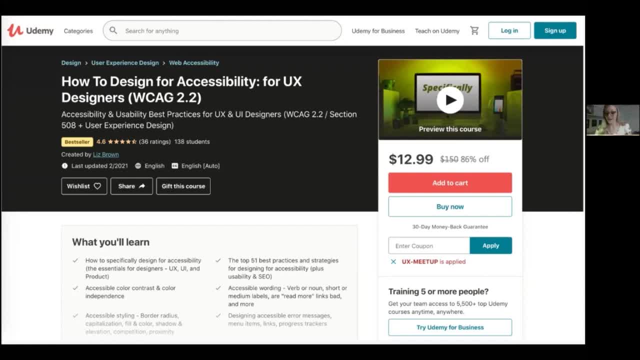 But so far it's been getting five stars, four and a half stars, So it really makes all this work I've put into it feel worth it. It took me- okay, this is a secret, you guys- It took me like ten months to make this. 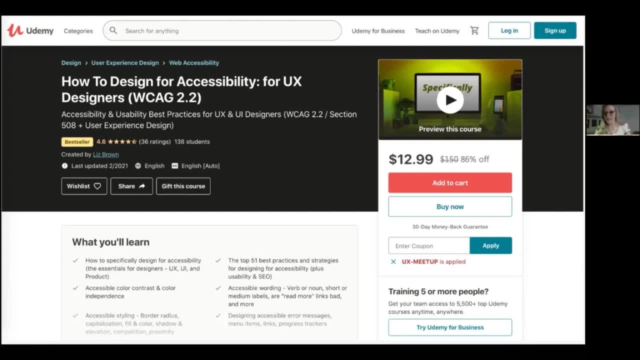 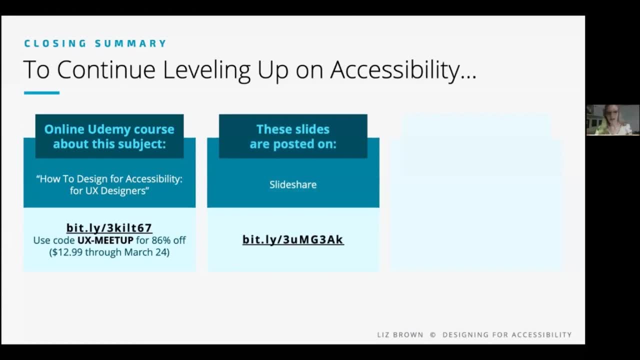 It's insane how long this stuff takes. So definitely take advantage of that coupon code if you're interested in becoming proficient in accessible design. The other thing: these slides that we looked at today. if you want to reference them later, I put them on SlideShare. 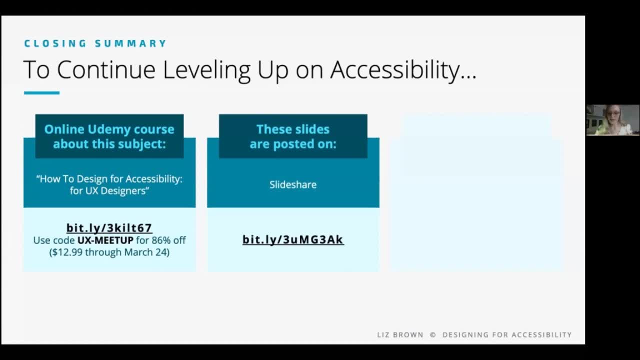 There's the link Again. I'll post these links in the chat here in a minute so you can pull them up in a new tab to look at after the call if you're interested. And then finally, the recording that Ben is doing. he'll put it on the Discord. 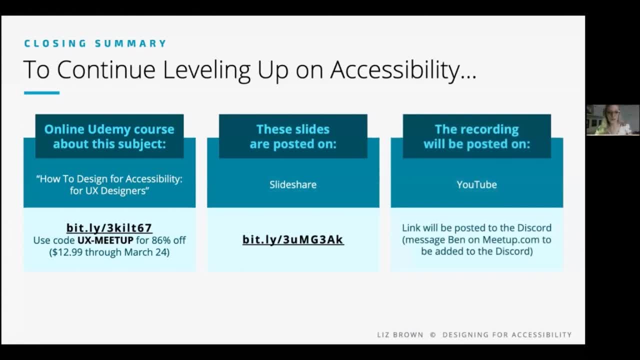 And if you're not on the Discord, just message Ben on muteupcom and he'll add you All right. So with that, are there any questions?